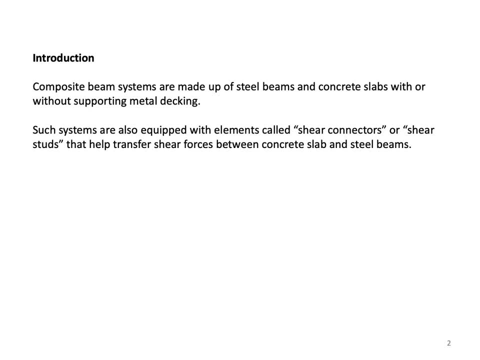 metal decking. Such systems are also equipped with elements called shear connectors or shear studs that help transfer shear forces between concrete, slab and steel beams. Composite beam systems are popular as floor systems in buildings and also in bridges. Design for a composite beam system includes proper 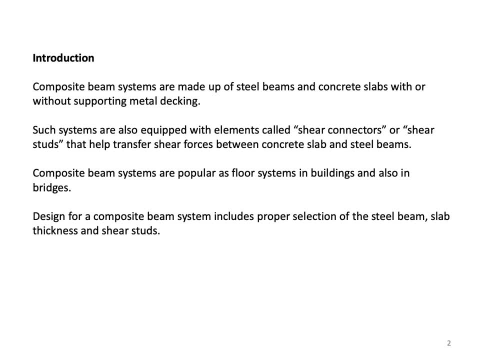 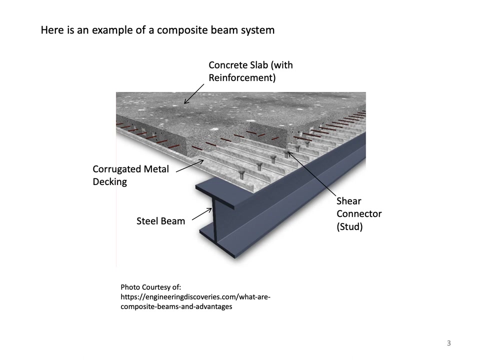 selection of the steel beam, slab thickness and shear studs. Shear studs are generally headed bars or pieces of channels that are welded to the top flange of the steel beam. Here is an example of a composite beam system. As you can see, in this special case, corrugated metal decking is used to support. 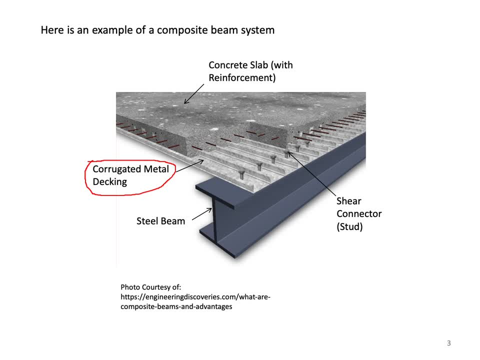 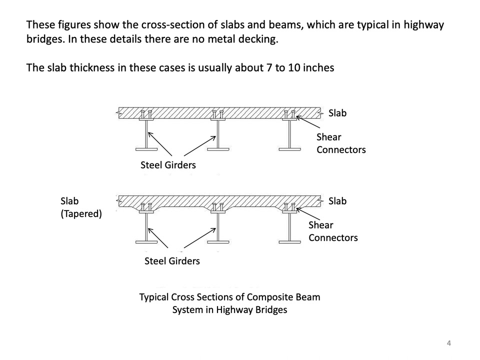 concrete. during construction, The concrete is reinforced. Metal studs are used in here. These are shear connectors And of course there is a steel beam and shear connectors are welded to the top flange of this beam. These figures show the cross section of slabs and beams which are typical in highway bridges. 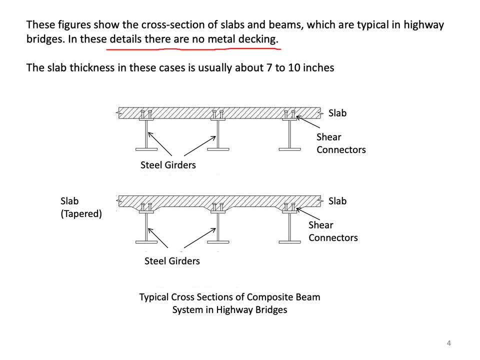 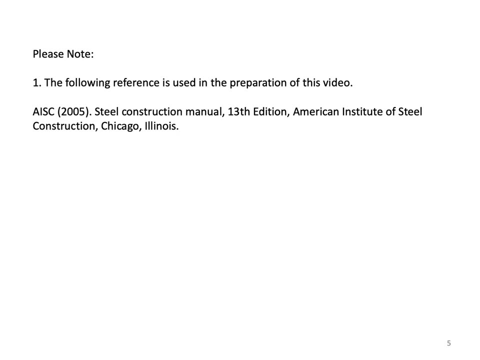 In these details, there are usually no metal decking And the slab thickness is about 7 to 10 inches. Please note that we are using the following reference in the preparation of this video: AIAC 2005, Steel Construction Manual, 13th edition published by the American. 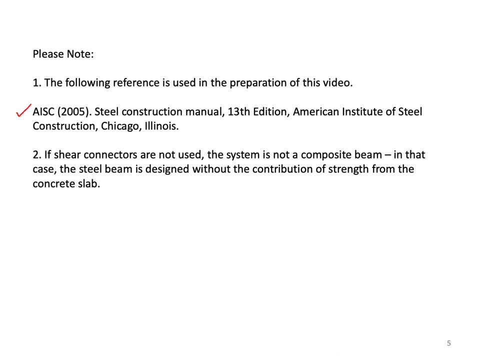 Institute of Steel Construction. Also notice that if shear connectors are not used, the system is not a composite beam. In that case, the steel beam is designed without the contribution of strength from the concrete slab. The slab design and its reinforcement is not covered in this video. The slab design follows. 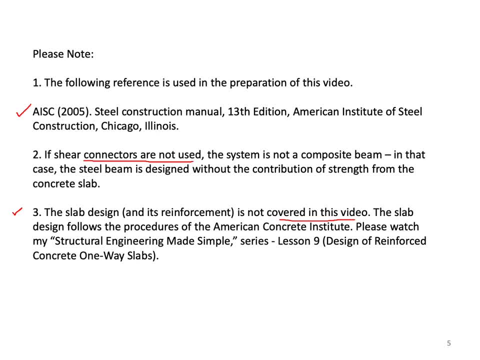 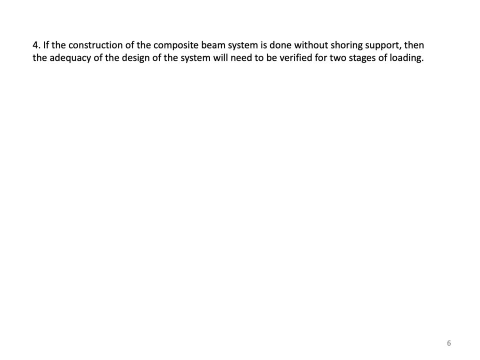 the procedures of the American Concrete Institute. Please watch my Structural Engineer Med Simple Series, which talks about the design of reinforced concrete one-way slabs. If the construction of the composite beam system is done without shoring support, then the adequacy of the design of the system will need to be verified for two stages of loading. 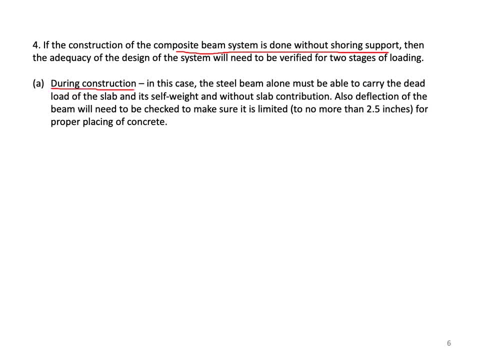 These are during construction. in this case, the steel beam alone must be able to carry the dead load of the slab and self-weight, and without a slab contribution. Also, deflection of the beam will need to be checked to make sure it is limited to no more than 2.5 inches. 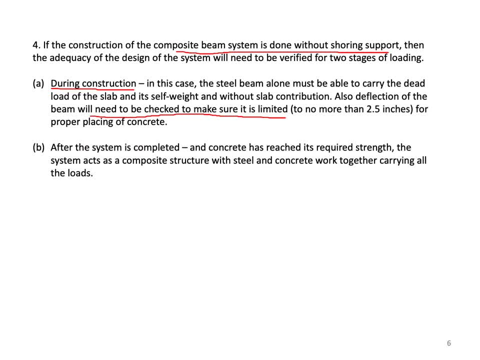 for proper placement of concrete After the system is completed and concrete has reached its required strength. the system acts as a composite structure with the steel and concrete work together now carrying all the loads- dead load and live load, both The live load deflection after the construction, and with the composite beam, action is limited to. 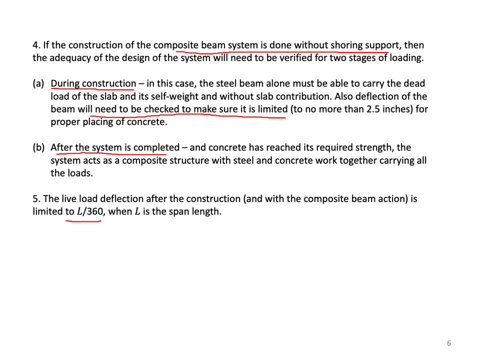 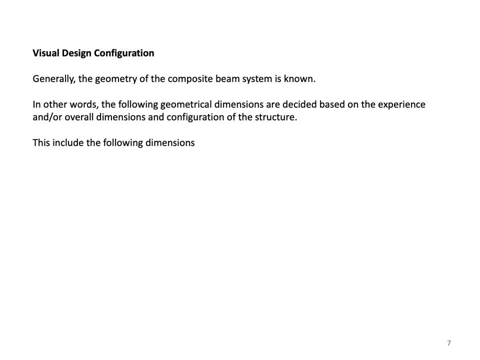 L over 360, when L is the span length. Visual design configuration. Generally, the geometry of the composite beam system is known. In other words, the following geometrical dimensions are decided based on the experience and or overall dimensions and configuration of the structure. 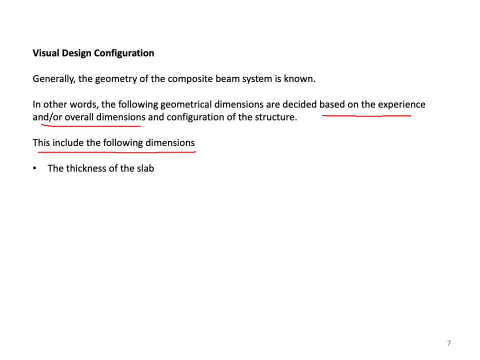 This includes the following information and dimensions: The thickness of the slab, If metal decking is used. the deck configuration, including the height of the rib, hr and its width. Now if, for example, we have a corrugated metal decking, we are talking about hr as a height and wr as a width. 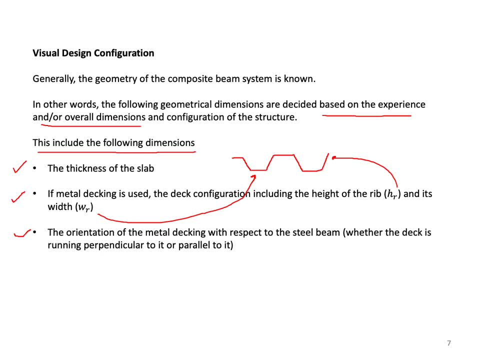 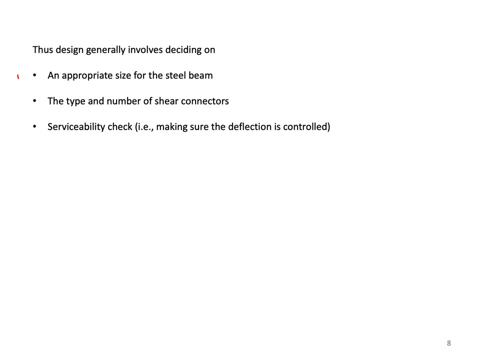 The orientation of the metal decking with respect to the steel beam, Whether the deck is running perpendicular to it or parallel to it, The spacing between steel beams. Therefore, design generally involves deciding on an appropriate size for the steel beam, the type and number of shear connectors and the serviceability check. 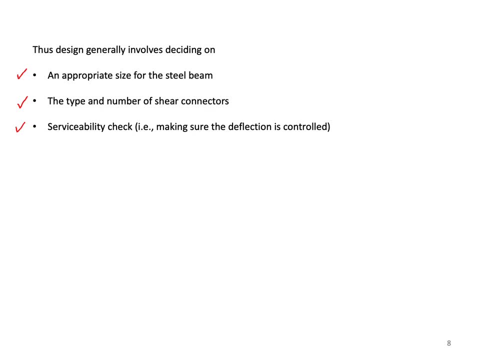 In other words making sure the deflection is controlled. A conservative design may be performed without design aids. However, generally, it is advised that design tables of the AIAC be utilized for proper design. In any case, it is important to know how to compute the moment. resistance of the composite section. 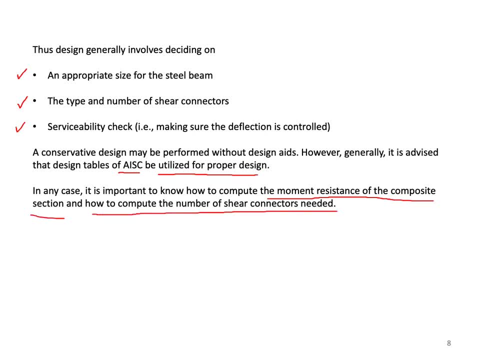 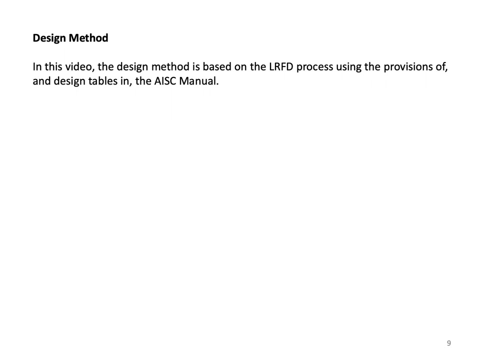 and how to compute the number of shear connectors needed. Depending on the number of connectors used, a full composite or partial composite action may be achieved. We're going to talk about this later Design method In this video. the design method is based on the LRFD process, using the provisions of 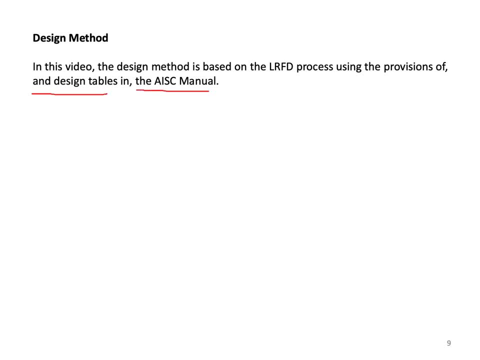 and design tables in the AIAC manual. Since generally the composite beam systems in buildings are designed for floor loads, the following two load combinations are considered in computing: the factored applied moment MU and factor shear VU: 1.4 times the dead load. 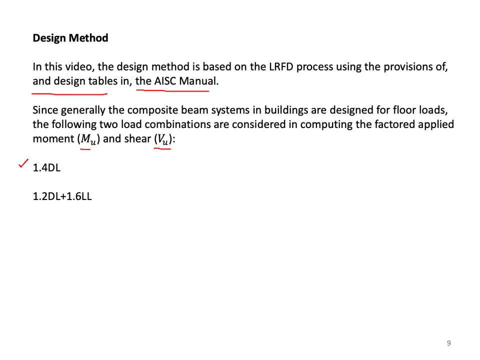 Usually this is during construction: 1.2 dead load plus 1.6 live load. Usually this is after the composite action has taken place For roofs. if a snow load is more critical than the live load, the load combination will be for the dead load and the snow load, with considerations. 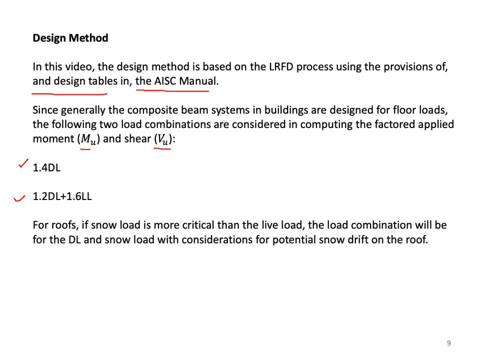 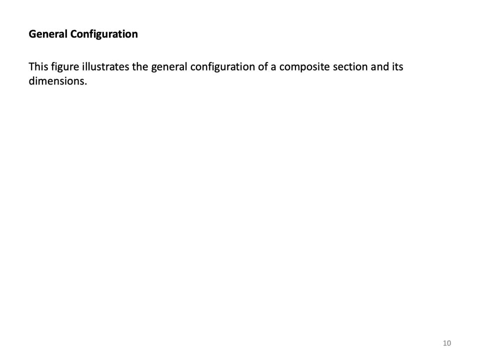 for potential snow drift on the roof. The snow drift would create some sort of trapezoidal or triangular distribution for the snow load. General configuration. This is the general configuration. This figure illustrates the general configuration of a composite system and the dimensions. 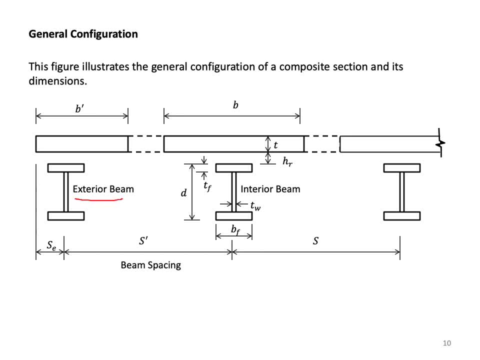 As you can see here, the distance between the exterior beam and the edge of the slab is designated as SE. The spacing between the beams is S, prime or S. Now, it could be the same or could be different. That's why I use S prime and S When it comes to deciding on the effective width of the slab. 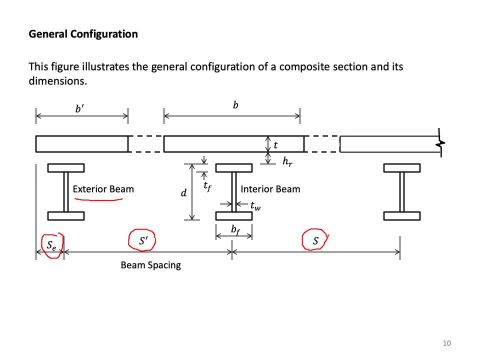 because not the entire width of the slab is considered. for the exterior beam. the effective width is B prime. for the interior is B, and let's see how we can compute them: B prime is the minimum of the edge distance SE and one-half of the spacing. 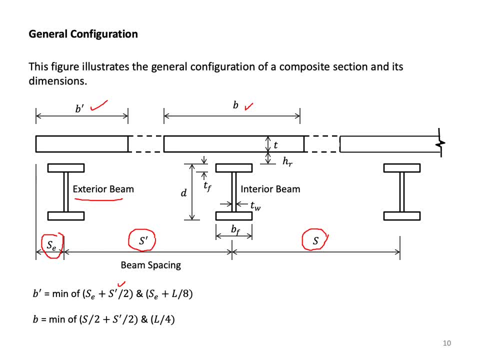 which in this case is S, prime and SE, plus one-eighth of the span length. L is the span length of the beam. However, for an interior beam, B is a minimum of half of the spacing from one side plus half of the spacing from the other side and a quarter of the length of the beam. 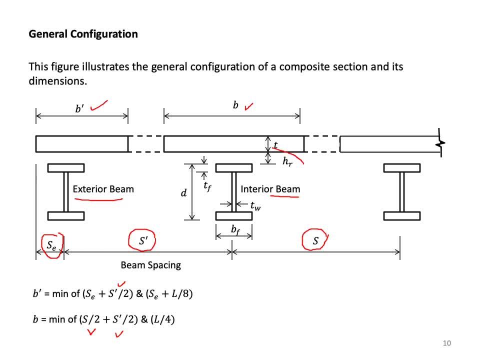 Also notice that in this configuration we have designated the height of the metal decking as HR, and if there is no metal decking, then of course HR is equal to zero. We need to know the thickness of the slab T and the properties of the section of the steel beam, including the width of the flange. 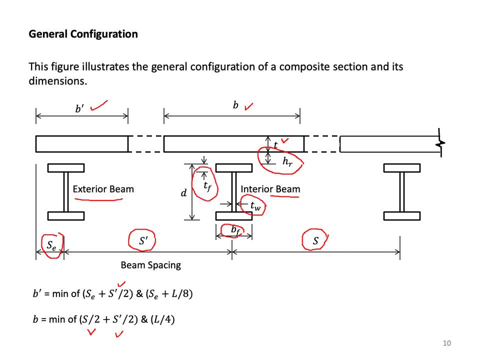 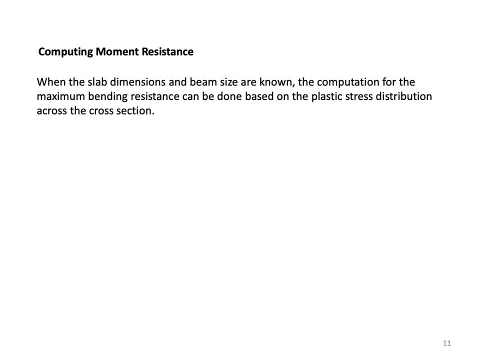 thickness of the flange, thickness of the web and so on. Computing moment resistance: When the slab dimensions and beam size are known, the computation for the maximum bending resistance can be done based on the plastic stress distribution across the cross section. Please note that certain requirement on the web slenderness ratio need to be satisfied. 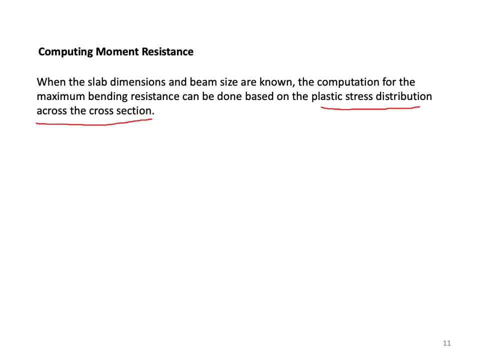 as I'm going to talk about later. so that we can use the plastic stress distribution, The nominal bending strength is designated as MN. The factor of the strength is phi B multiplied by MN. Phi B in this case is 0.9.. 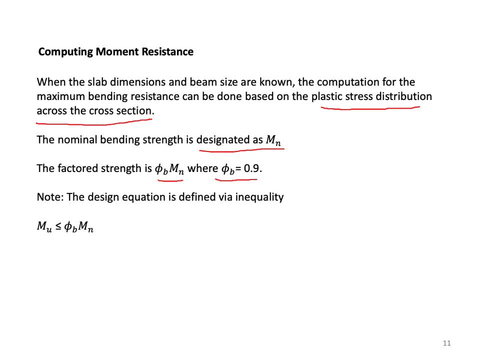 It is the resistance reduction factor. The design equation is based on the inequality MU smaller or equal to phi B, MN, where MU, as you realize, is the factored applied moment and MN is a nominal resistance. There is a similar equation for shear. 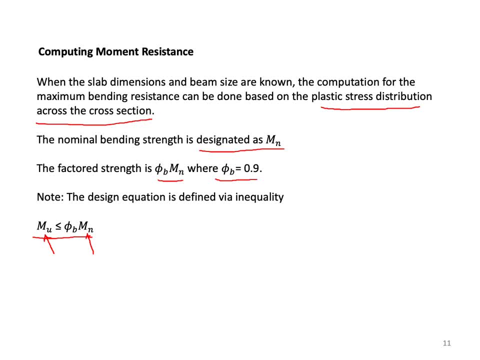 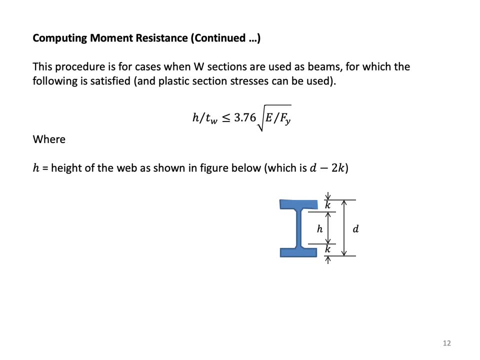 But in this video we are not talking about shear. I'll just make a reference to it. This equation is based on the inequality of mu, which is equal to phi B, MN, and MN is a nominal resistance And phi B is the shear, which is a moment resistance. 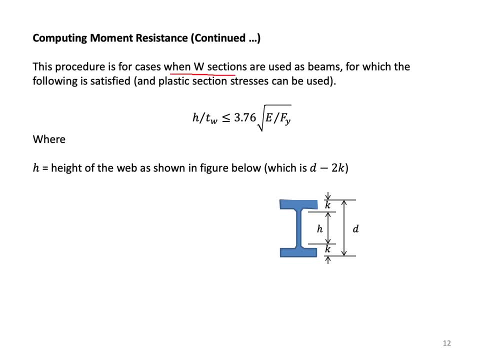 And phi B is the shear, which is the moment resistance, And phi B is the shear, which is the moment resistance. This procedure for computing the moment resistance is for cases when W sections are used as beams, for which the following equation is satisfied: 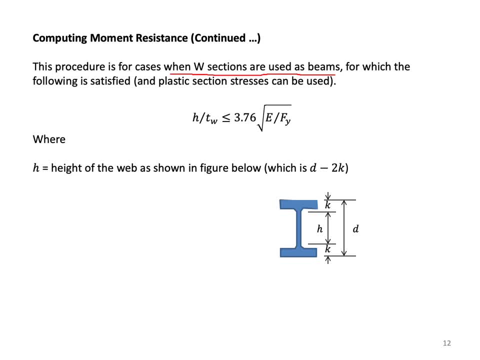 This is H over T W. This is the slenderness of the web and it is smaller than 3.76 times the square root of E over phi. E is the modulus of elasticity of steel and phi is the yield capacity of steel. 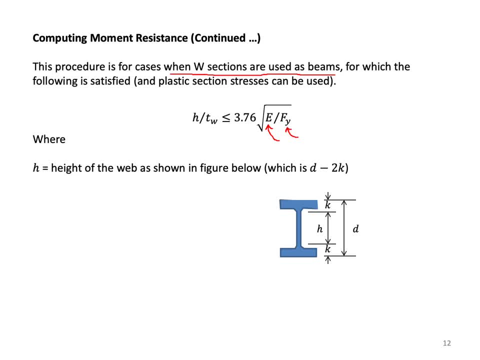 which is for W sections 50 ksi. The parameter h is the flat portion of the web. as you can see, here is d minus 2 times k, and these values are all listed in the AIEC manual for different sections. 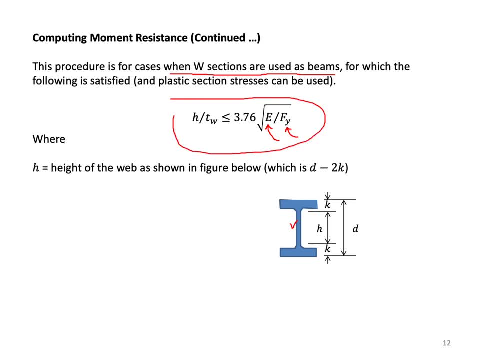 For W sections. this inequality is always satisfied In cases when h over TW is larger than that limit. AIEC requires using superposition of elastic stresses with the effect of shoring for the limited states of yielding. The moment resistant in this case is the yield moment And there is a procedure for computing the moment resistance. 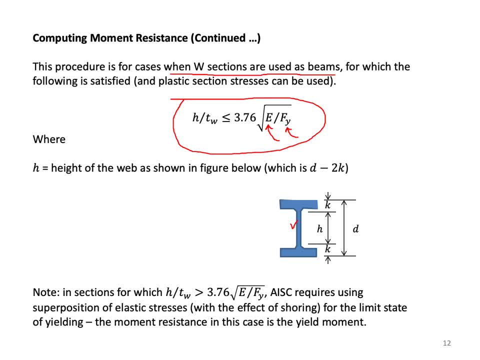 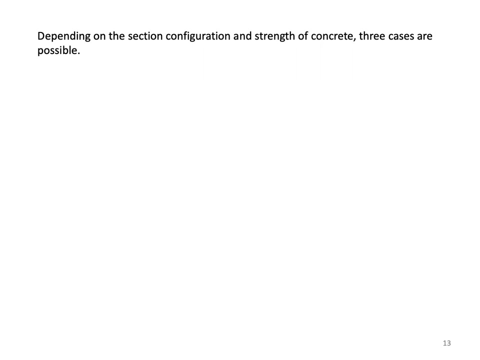 Usually you need to use what we call transformed beam and I'll talk about that towards the end of my video. briefly talk about how you can find the transformed section and get the properties of the section accordingly and compute the moment resistance Depending on the section configuration and the strength of concrete. three cases are possible. 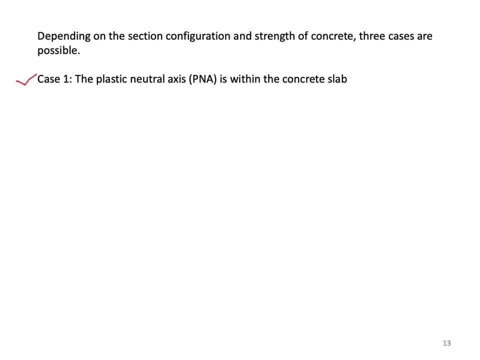 Case one: the plastic neutral axis P and A are the same as the plastic neutral axis P and A are the same as the plastic neutral axis P and A are the same as the plastic neutral axis. P and A is within the concrete slab. Case two: the P and A is within the top flange of the beam. 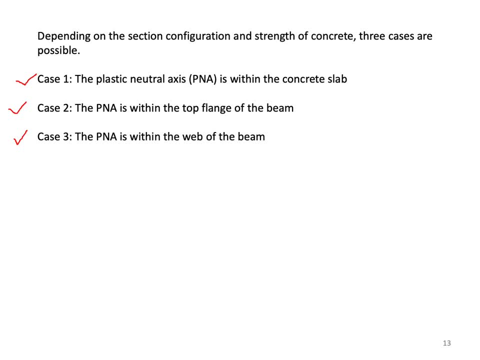 Case three: the P and A is within the web of the beam. For a given composite section, we can find out which condition governs To do that. first we need to compute the maximum compression force on concrete- I call it Cmax- and the maximum tension. 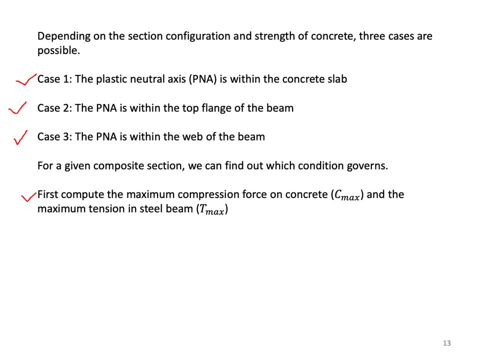 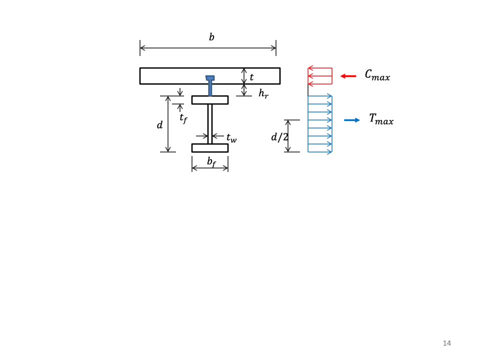 in the steel plate, which is the maximum compression force on concrete, I call it Cmax, and the maximum tension in the steel plate, which is the maximum tension in the steel plate, we call it Tmax, Cmax and Tmax. So here is the configuration. As you can see here the dimensions are given. 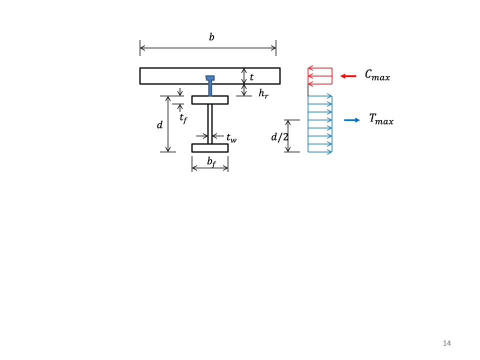 In this condition, when we want to find the Cmax we are considering, the entire slab is under compression with the stress of 0.5 of prime sub c and the entire steel section is yielded with the yield capacity Fy. Therefore, Cmax is simply the area of concrete, which is B. 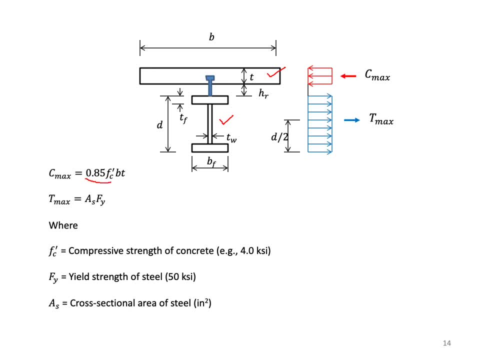 times T multiplied by 0.85 of prime sub c and for the Tmax is the area of steel multiplied by Fy. If prime sub c is a compressive strength of concrete, usually around 4 ksi or 3 ksi, Fy, as I said, yields the strength of steel or yield capacity of steel, which is 50 ksi for W. 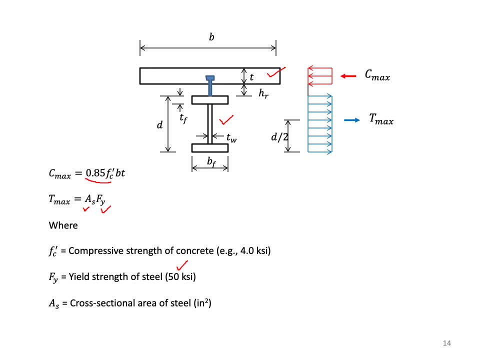 sections and As is a cross-sectional area of steel which is in square inches. Now, if you are talking about an existing, let's say, floor system which is 50 years old, or maybe 40 years old, and you are computing the strength of the composite section, chances are the W sections that are used. 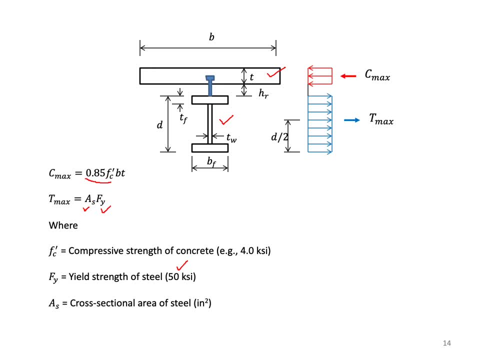 have an Fy of 36 ksi And if you compute the strength of the composite section, chances are the W sections that are used have an Fy of 36 ksi. So you need to know from the marking on the sample or the beam what kind of yield capacity they have. 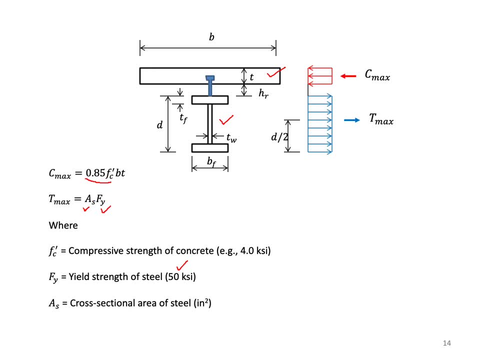 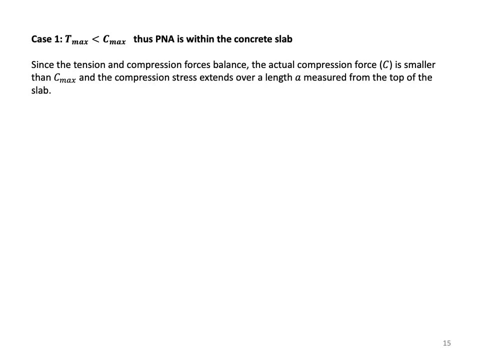 But most current steels W sections have 50 ksi of yield strength. Case one is when Tmax is smaller than Cmax. What happens if Tmax is smaller than Cmax? Well, that means the smaller compression force is needed to balance with the tension. 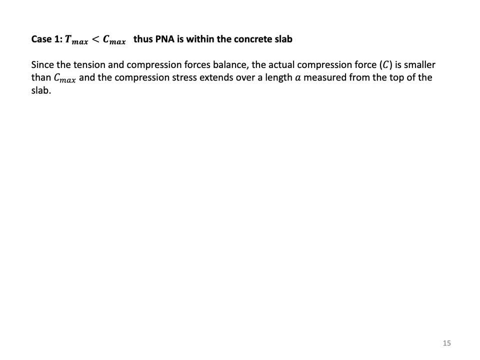 Therefore, the P and A would move up, So P and A would be within the slab. Let's look at the configuration. So here is the situation. You notice that the area which is shaded by red, that's where the compression force is. 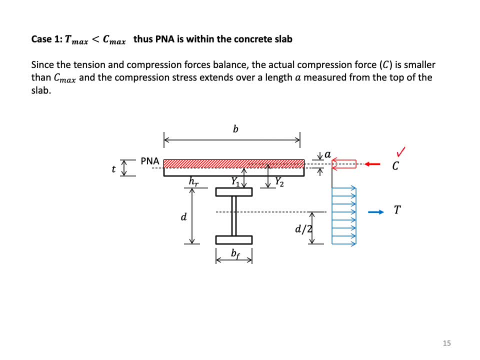 Now the compression force is. C is smaller than Cmax, However the tension is lower, So the tension force is still As multiplied by Fy. You notice that the depth of the compression is shown with a little a And the location when the force C applies is halfway from the top in distance A. 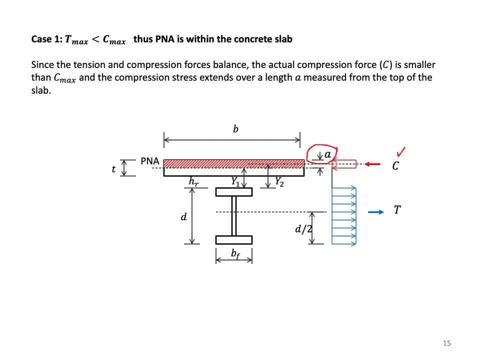 In other words, it's at A over 2 from the top. However, just following the AISC procedures, we identify two dimensions: Y1. And Y2.. Y1 is a distance between the plastic neutral axis P and A to the top flange of the steel beam. 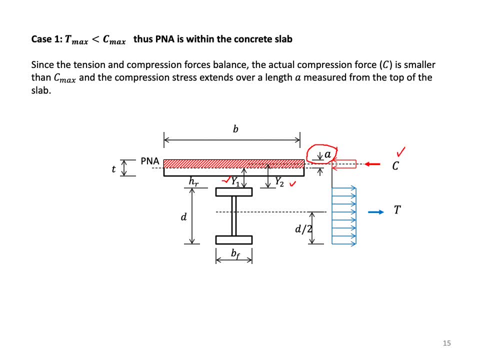 And Y2 is a distance between the location when the compression force C applies to the top flange of the beam. So in this special case Y1 and Y2 are slightly different from each other. This line in here is the top flange of the steel beam. 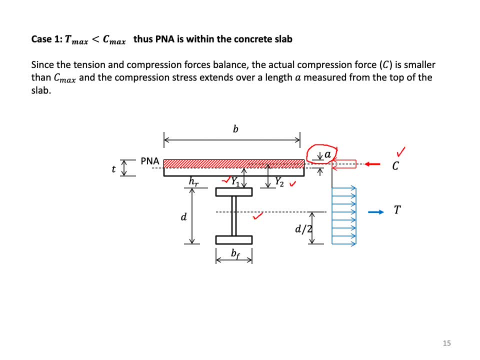 And Y2 is the distance between the top flange of the steel beam And Y2 is the centroid of the steel beam And in this video I'm going to use that one as my reference point, Although depending upon the values of the load and the location of P and A. 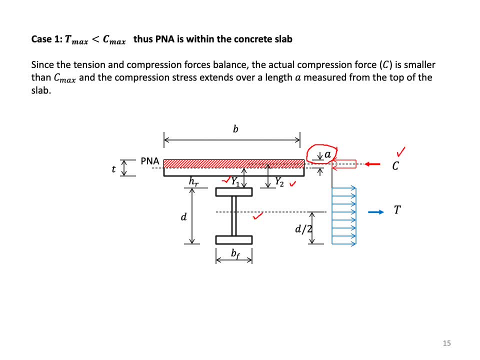 the plastic neutral axis may be, as you can see here, way up or way down, But the resultant for the tensile forces not always fall under this line. So I'll talk about it later and you will see what is involved. But you can very conveniently use this line as your reference line. 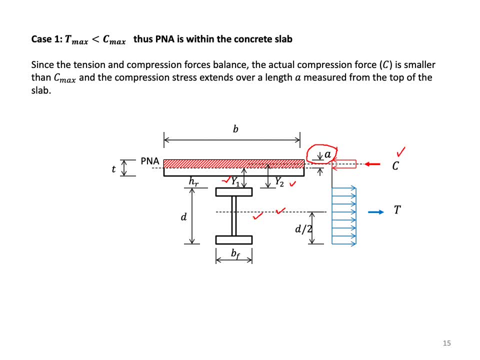 in computing your moment for finding the MN. All right. So, as I said, Y1 and Y2 are the two dimensions that we are following the AISC manual for those And just looking at the geometry we notice that therefore, Y1 is HR plus T minus A. 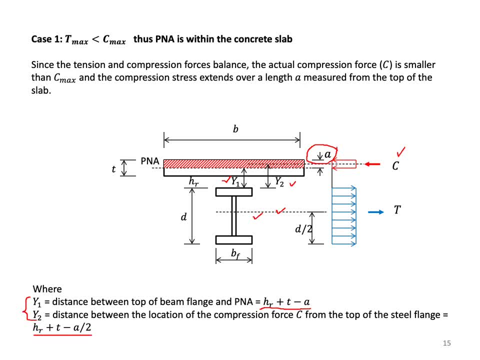 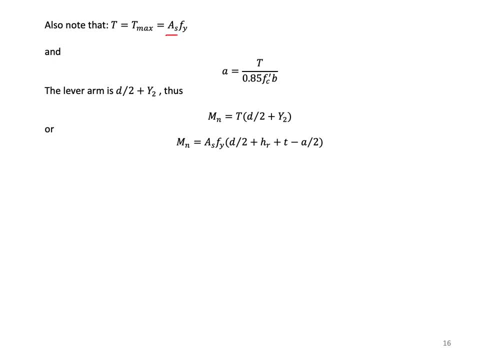 However, Y2 is HR plus T, minus A over 2.. Because T is equal to T, max is AS over FY. with the balance of forces, writing in other words the tension equal to compression, we can get an equation for A: A is equal to T, which is ASFY divided by 0.85. prime sub CB. 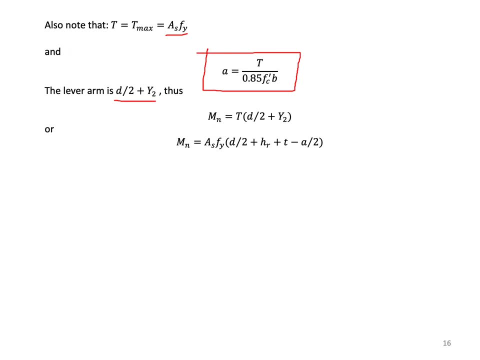 The lever arm is D over 2 plus Y2.. Remember that I said the centroid of the steel beam is my reference point. Therefore, the moment is simply T times D over 2 plus Y2, or, if you want to substitute Y2,: 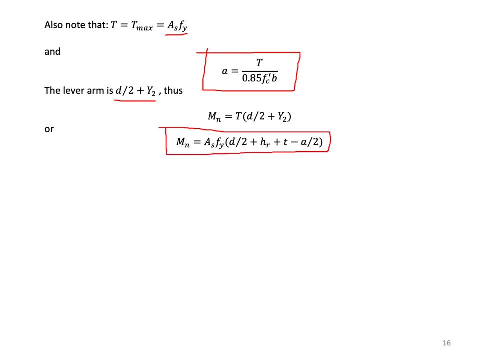 this is the equation you get for the moment: resistance, So a pretty straightforward in this case. Then the next question is how many shear connectors I need For that? I have two connectors For that. we need to find the horizontal shear force at the top flange. 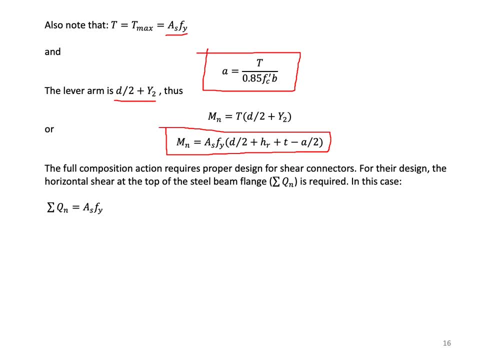 because that's where the shear connectors are connected to the steel And for that again from the plastic stress diagram, and you can simply start from the bottom of the section and go up and find out how much force you have in this special case. 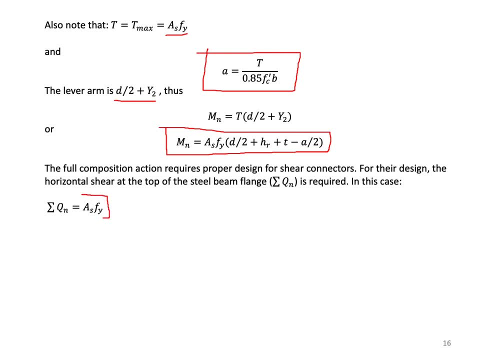 You notice that, therefore, the total force is AS times FY And AISC. you have to find the shear force And AISC uses the designation sigma QN. Sigma QN is the horizontal shear at the top of the flange. 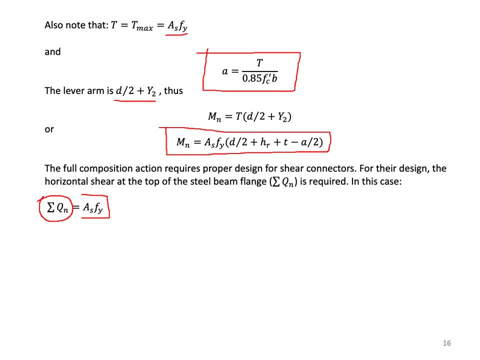 We need that shear to compute how many shear connectors we have. So if the resistance of one shear connector is QN, just one, therefore the total number would be the shear force sigma QN multiplied by QN. Right Now sometimes you use double starts, two together. 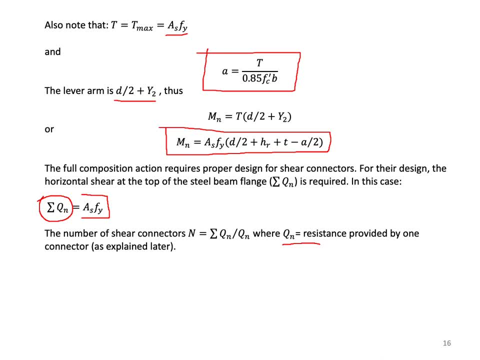 In that case, of course, usually we need to multiply the QN by two when we put it in this equation. So I'll demonstrate that for you in an example problem later. Shear connectors are distributed at equal spacing between the point of zero moment. 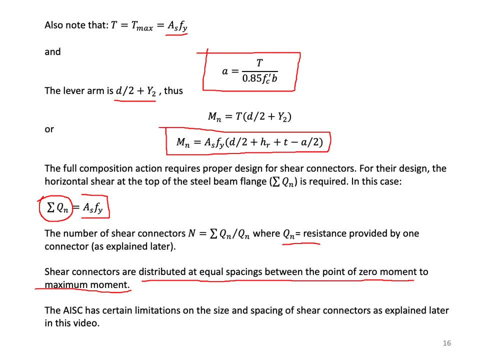 to the maximum moment. And please note that point of zero moment to point of maximum moment is actually where the shear is zero and the shear becomes maximum. So for a simply supported beam, this would be from one end of the beam to the mid-span of the beam, right for half of the beam. 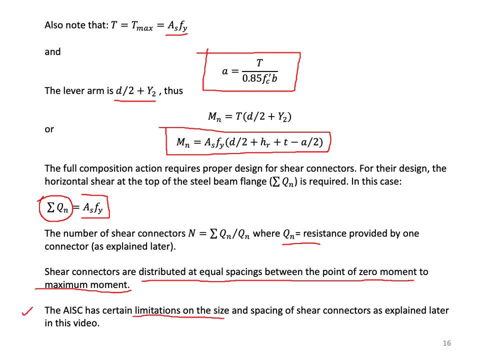 Also, please note that AISC has certain limitations on the size and spacing of shear connectors, As we explained later in this video, And also there is some requirement on the height of the connectors. The connectors need to be about one and a half inches at least above the top. 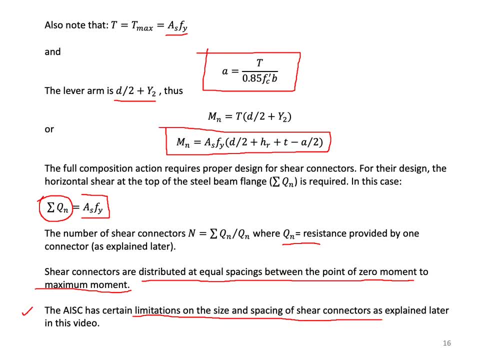 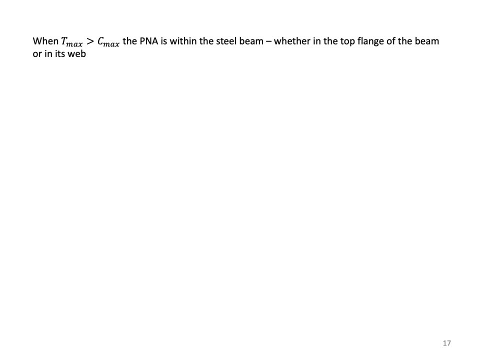 of the metal decking. if metal decking is used And the concrete cover needs to be at least one and a half inches above the top of the shear connector. All right Now, if T max becomes larger Than C max, the plastic neutral axis is within the steel beam. 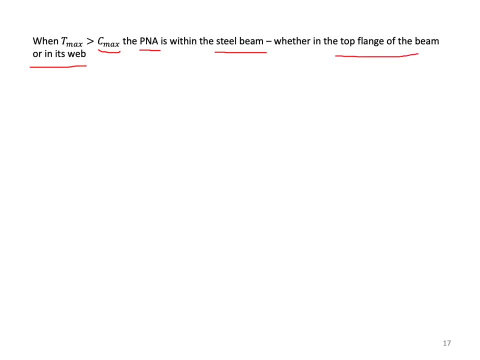 Whether in the top flange of the beam or in its web. Now let me talk about why we get into this situation first. Sometimes the beams are much stronger than the slab. For certain reason, we have to use a very strong beam and very small slab. 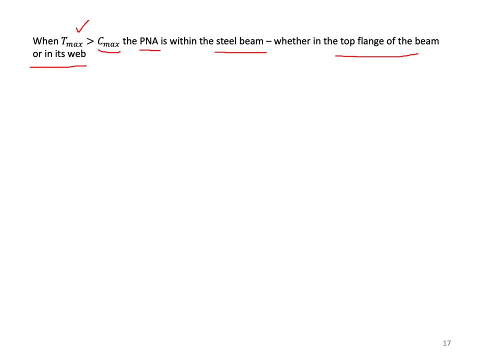 So this condition may happen. Other areas This condition may happen is when we don't have the full composite action, We just have partial composite action, And in that case it all depends on how many shear connectors you use. The less number of shear connectors cause the partial composite action. 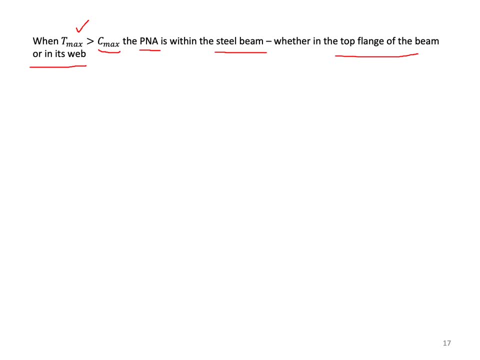 Now, if you need to have a complete discussion on full, partial composite action or partial, Or full composite action or partial composite action, I suggest that you look at the textbook in steel design. So let's look at case two. when PNA now is in the steel beam, however, is in the top flange of the steel beam. 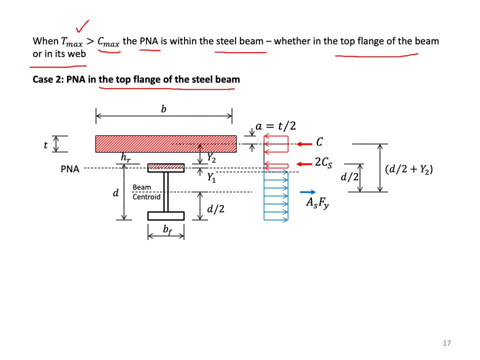 And this is the pertinent diagram that shows the distribution of plastic stresses. Now you notice that the concrete slab right now is completely loaded because the PNA is much below. The small portion of the top flange of the beam is now under compression. A red shaded area means compression. 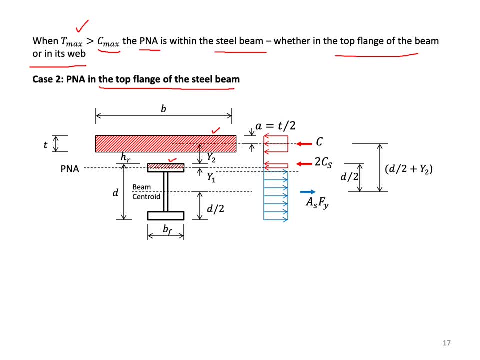 So we have a force C and we have a little force C sub C, which is the compression on steel. C sub S, rather So C sub S. Why do I put two C subs S? I'll talk about that later. And for the tension force I put ASFI. 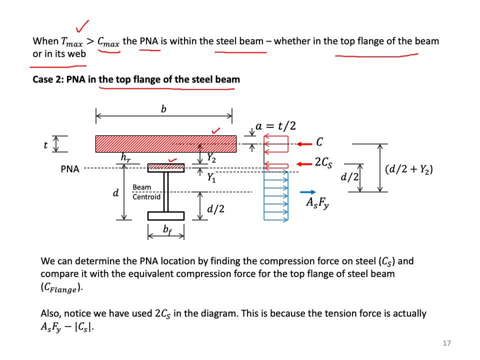 but it's actually not ASFI, because not the entire beam is under tension. A small portion at the top is under compression. Therefore, I need to deduct from ASFI an equal amount Cs to have the total force. However, for the convenience, 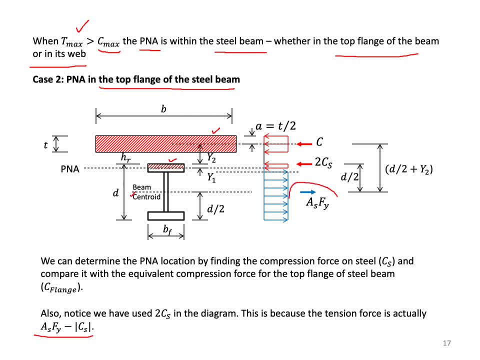 in order to use the beam centroid. I still use ASFI And that Cs that I need to deduct from this, I put it up here. That's what I get: two Cs. So this is how I would show the diagram And I think the computation of MN is much easier. 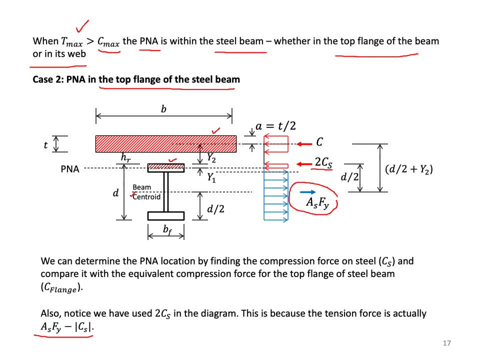 But there is another way that most textbooks talk about it. I'll tell you about it later. Now you notice that Y2 is changed because it's from the top of the flange to the center of MN, The center of this slab, because that's where the load C applies. 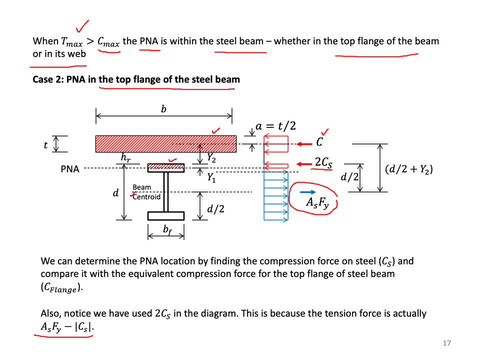 And the Y1, which shows the location of PNA, is a small Y1, is the distance from top flange to PNA. Alright, So the distance between force C and, if we use our reference line as beam centroid, that is D over 2 plus Y2.. 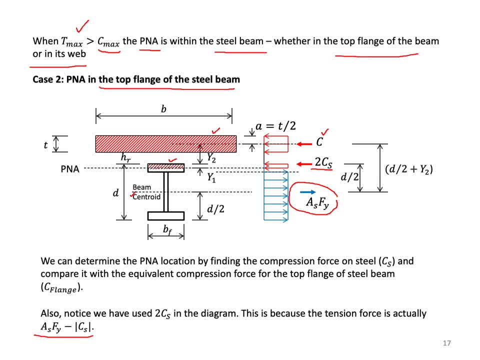 Keeping that in mind, and let's now continue with our calculations. And I also introduce a new parameter called C, flange, And that is the compression force, if the entire flange were under compression. But you notice not the entire flange is under compression. 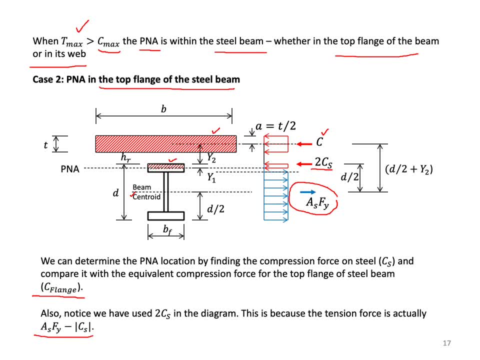 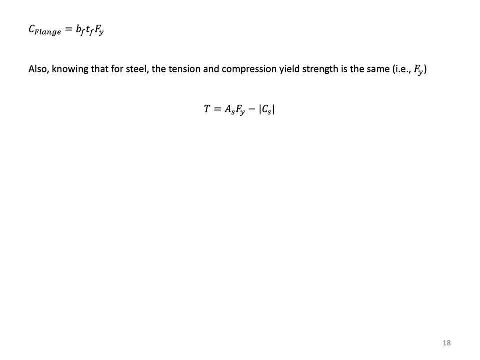 It's just a portion of it, But if the entire flange is under compression, I can find that value very easily. I call it C flange. Okay, So what is C flange? That would be the width of the flange times thickness of the flange. 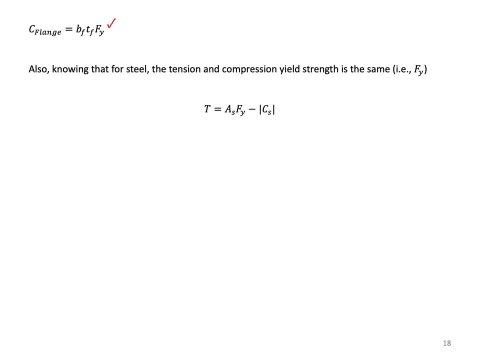 multiplied by FI. Keep it handy. We'll come back to this later. So remember that I said the tension force is FI minus CS. But why am I using the absolute value of CS? Well, it doesn't matter, You can simply use CS. 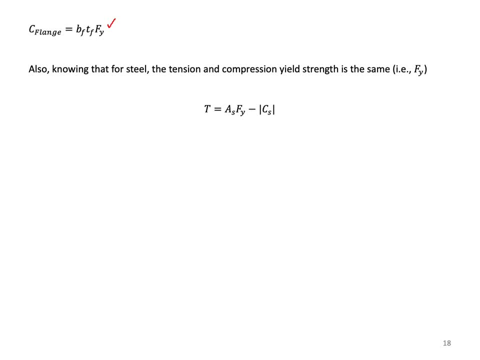 The reason I'm using absolute value is because some people would like to use a sign convention for compression and tension, And I just want to say that do not use any sign for CS, Just use the same value as CS that you get. That's the only purpose. 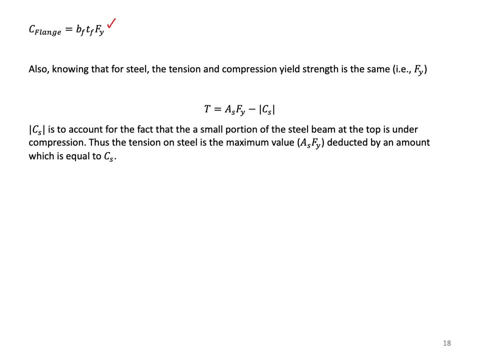 All right Now, as I said, CS is to account for the fact that the small portion of the steel at the top is under compression. Therefore, the tension on a steel is a maximum value, ASFI, deducted by an amount which is equal to CS. 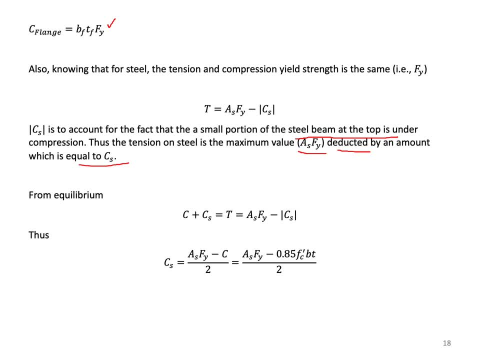 So writing: the equilibrium compression forces is equal to tension forces. Getting rid of the absolute value signs and solve this equation for CS, you get the value of CS computed, It's ASFI minus point A5, prime, sub C, BT, That's the compression force. 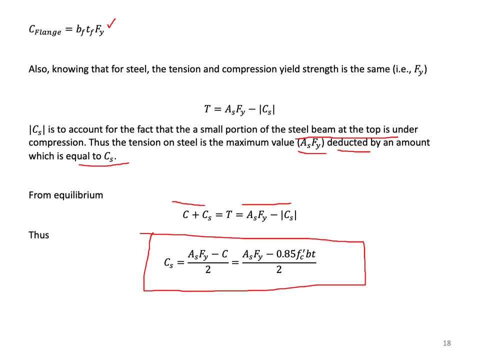 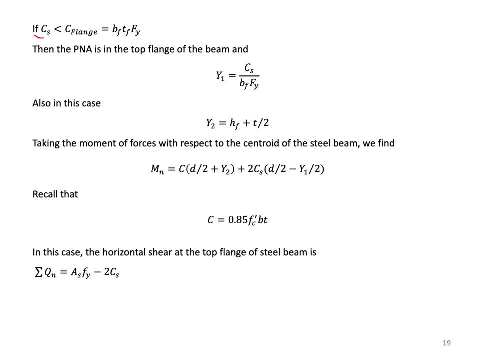 C divided by two. All right. So with this now we compare it with the C flange. If CS- that we just computed- is smaller than C flange, that means PNA is in the top flange of the beam. 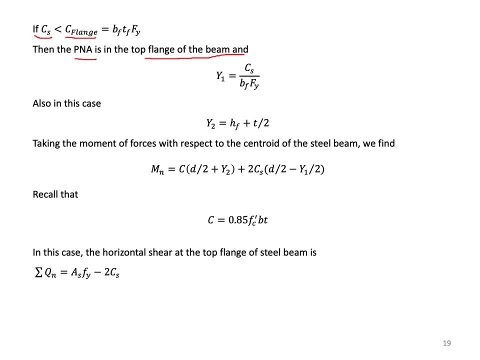 And we can very easily find, therefore, that Y1 that we were looking for, that CS divided by BF- that's the width of the flange- and FY, And now I have both Y1 and Y2.. Y2 is HF plus T over two. 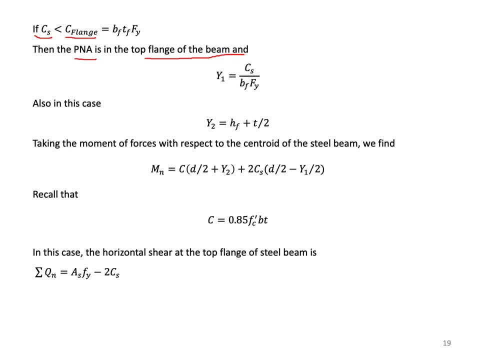 because the point of application of the compression is at T over two. And take the moment with respect to that reference line I told you about, So you get the force C multiplied by D over two plus Y2, two times CS multiplied by D over two, minus Y1 over two. 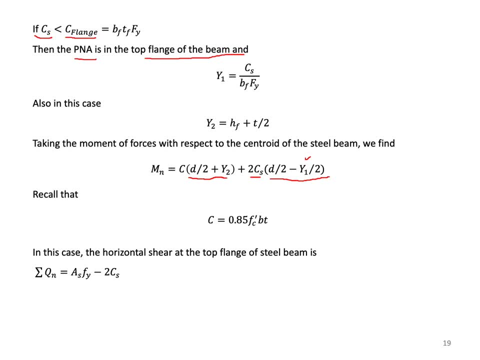 Where is this Y1 over two involved? Because the center of the application of CS is right at the center of the little area. And don't forget that C is equal to this value. So with that, the only other things left to determine is: 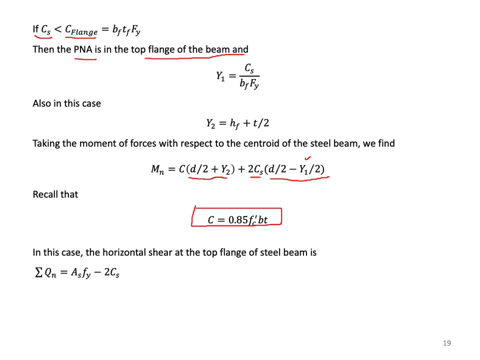 what is that? horizontal shear, Horizontal shear now is sigma QN, which is ASFI minus two CS, Because the tension force is ASFI minus CS and there is another CS as a compression, so we get two CS in there Again, if you want to find this. 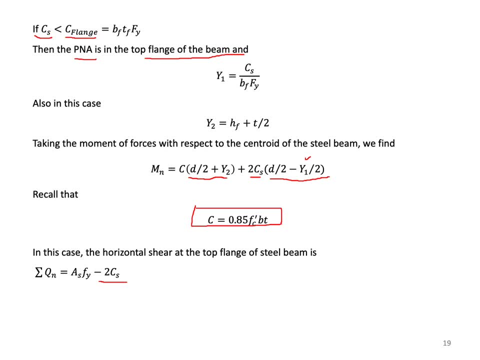 and don't want to memorize any equation. just start from the bottom and add all the forces Once you hit the top flange of the steel. that's where you have the shear force And, by the way, this is based on plastic stresses. 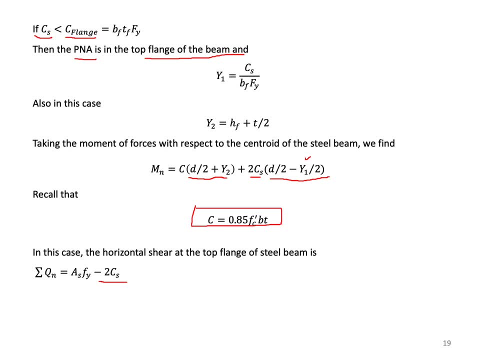 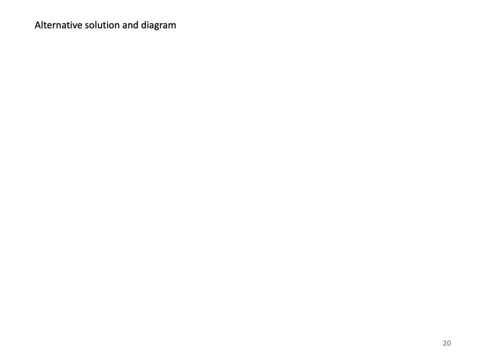 The traditional equation VQ over BI for horizontal shear stress. that is applied to elastic condition, not to this. For this one, you need to use this value, And I told you there is another way of showing the diagram Which most textbook use. 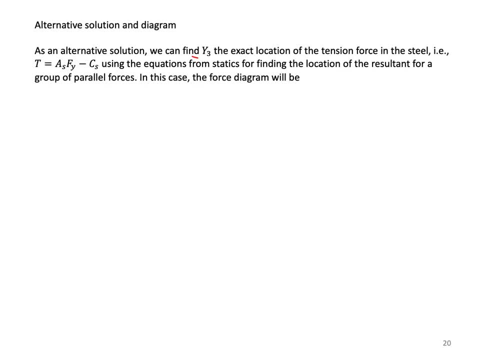 So in that case, what we do? we find another parameter which is called Y3. And for computing that we use the actual tension force, which is ASFI minus CS, And then we try to resolve all the vectors that show forces. 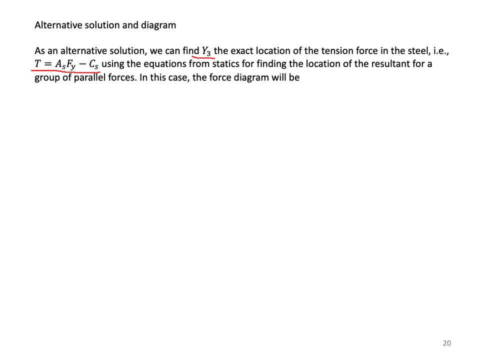 to figure out where is the exact location of this ASFI CS. It is not at the centroid of the steel, So it is different from that location, but we can find it. So let me show you the diagram and see how the diagram would look like in this case. 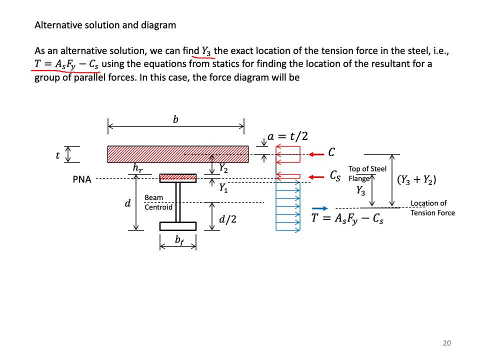 Well, you might say this is exactly like before. No, it is not, Because you notice that I only have one CS in here And I use this: deduct the CS from ASFI. This is the actual T And you notice it is not in this location. 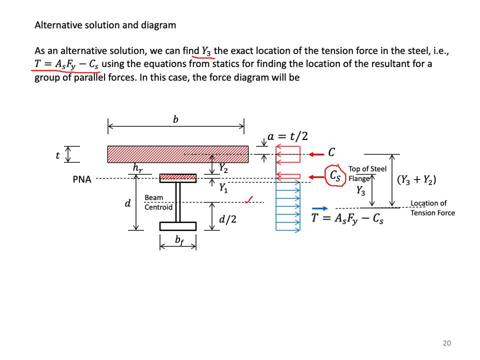 It is lower And it's actually at the distance Y3 to the top flange. So this is what I'm looking for. How do I find this? Well, you resolve, You know from statics. you have a bunch of vectors. 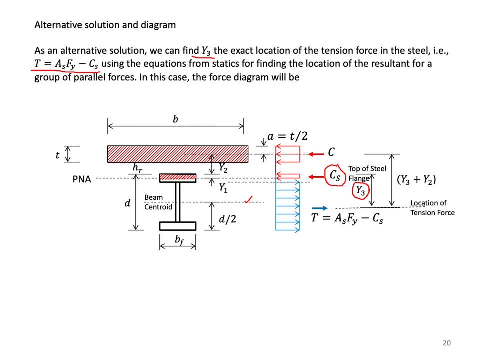 parallel to each other. You can find the resultant of those and you can find the exact location. So if you work your calculations, you come up with an equation for Y3. And in that case we use this point as a reference point to find the moments with respect to this point. 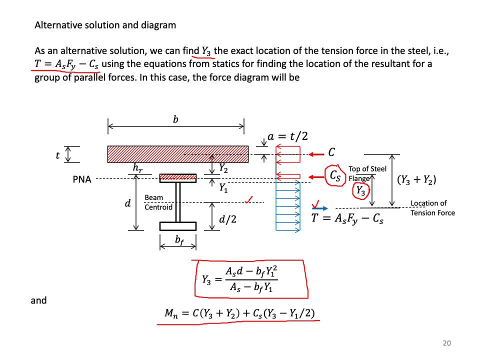 And we get this equation. for Mn, You get exactly the same value as before. If you look at a textbook in a steel design, you probably see this equation, But I think the previous one is easier, as long as you understand why it is 2CS. 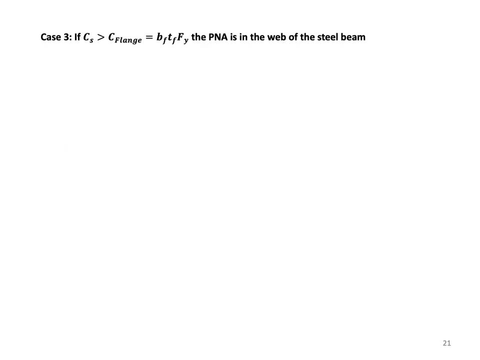 All right Now, if CS is larger than C flange, obviously that means the PNA is now moving further down. The PNA is in the web of the steel beam And I'm going to introduce two new plans and two new parameters. 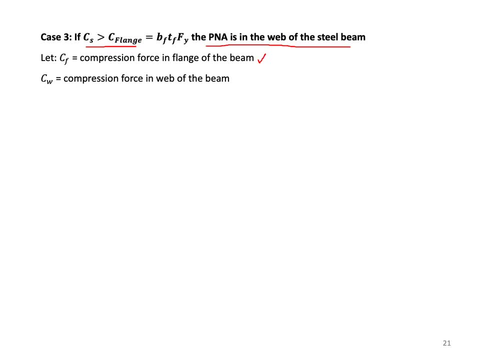 One is CF. Actually, this CF is the same as C flange. This is the compression force in the flange of the beam. It's the same as this value. I'm going to introduce a new value called CW, which is the compression force in the web of the beam. 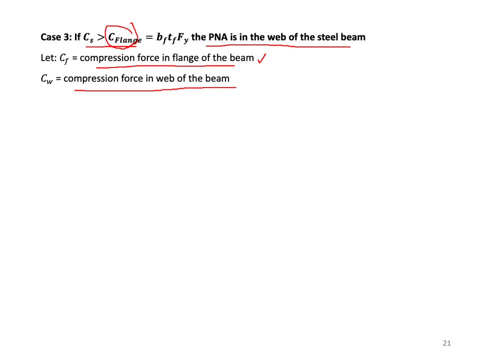 that little area that is under compression. Let me show you a diagram. You will see it much better what's going on. Very similar to the previous diagram, except that it is a small portion here which is under compression And I'm going to use a new parameter, Y3. 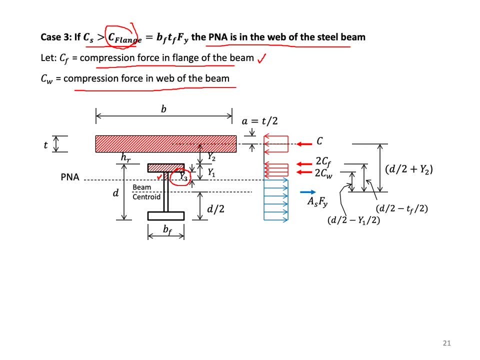 to show you that what is this area, In other words, to what extent this compression has gone into the web. That's the PNA, So similar before. if I use ASFI, show it at the centroid, then rather than a CW, I have 2CW. 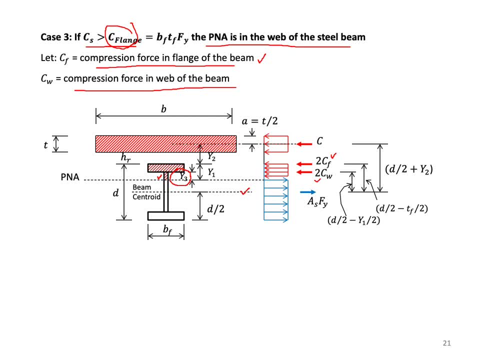 And rather than CF, I have 2CF, Because the actual tension is ASFI minus CF, minus CW. Very similar to the previous one, except that the CW is now added right And the Y3 represents the portion of the web that is under compression. 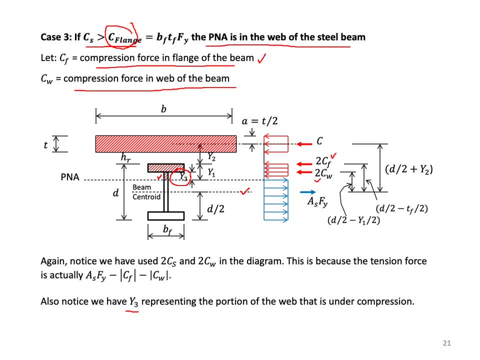 So all the other dimensions could be written. Y1 and Y2 are very similar to before. As usual, Y1 is the distance from the top flange to the PNA And Y2 is the top flange. the distance from the top flange. 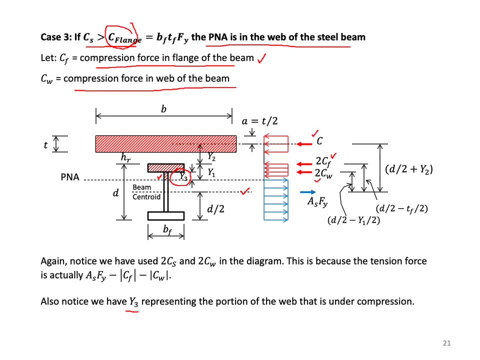 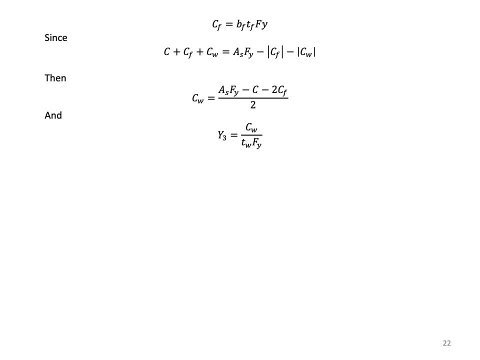 to the center of the application of the compression force. The next step is to go ahead and write the balance of the forces, all the compression forces equal to all the tension forces. From there you find the CW, And now you can get Y3,. 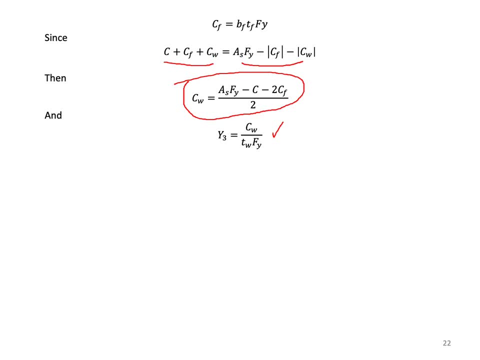 which is CW, divided by the thickness of the web and by the yield capacity of the steel, And take the moment of all the forces with respect to that centroid and you come up with this equation for the moment, resistance in this special case, And as a reminder, 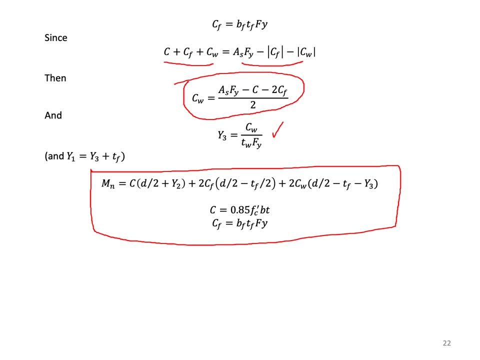 I wrote what C and CF are. Okay, Now the horizontal shear. By now you notice that it is the tension force which is ASFI minus 2CF, minus 2CW, right at location. the tension forces right at the location. 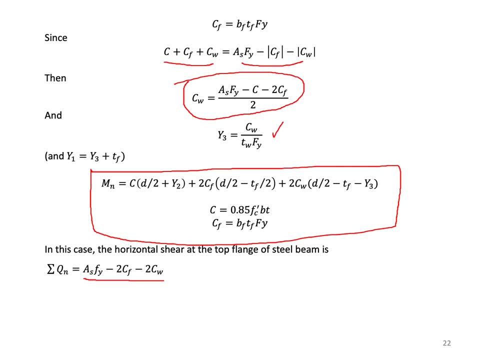 of the top flange. That's where this value would be equal to the horizontal shear. Okay, So is there, just like previously, an alternate solution? Yes, You can resolve the forces again using the equations of statics and you can find out exactly. 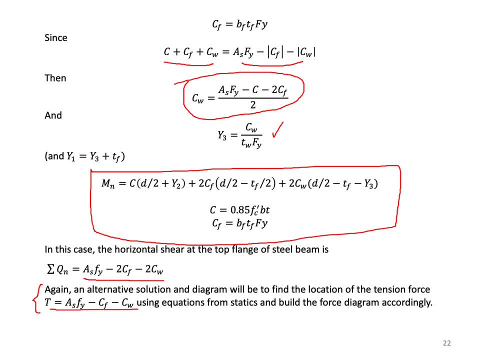 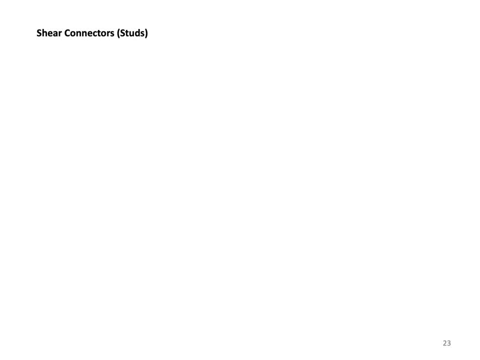 where this force, which is this is the actual tension- is located, and you can write a comparable equation for MN. Now let's talk about shear connectors. Shear connectors are in the form of headed bars or pieces of channels welded to the top of the flange. 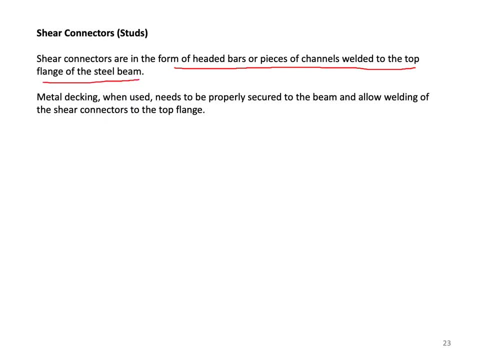 of the steel beam. Metal decking, when used, needs to be properly secured to the beam and allow welding of the shear connectors to the top flange. That's important. They need to be welded to the top flange of the beam. The strength of a headed bar. 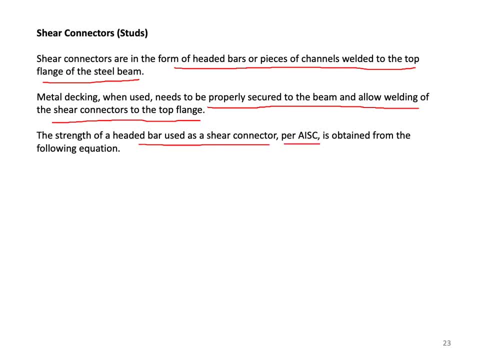 used as a shear connector per AISC is obtained from this equation. This has two terms in it. The first term is related to concrete: the area of the stud multiplied by this factor, which is property of concrete, and this is related to property. 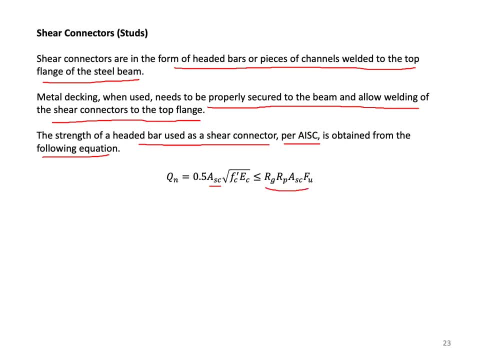 of the stud itself. Again, AISC is the area, Rg and Rp are two factors. We talk about that- And Fu is the ultimate strength, tensile strength of the stud, Because there are modes of failure, that one is related to crushing of concrete. 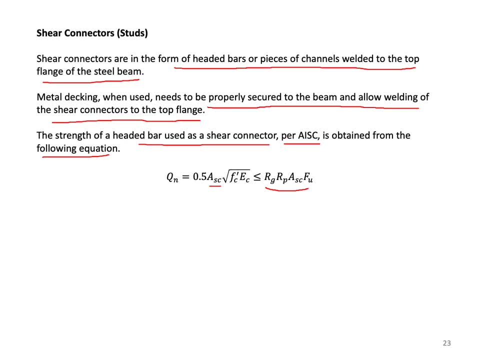 the other one related to the ultimate tensile failure of steel. We have to figure out which one is smaller. All right, AISC is a cross-sectional area of the connector in square inches. For example, if you use a half an inch diameter connector, 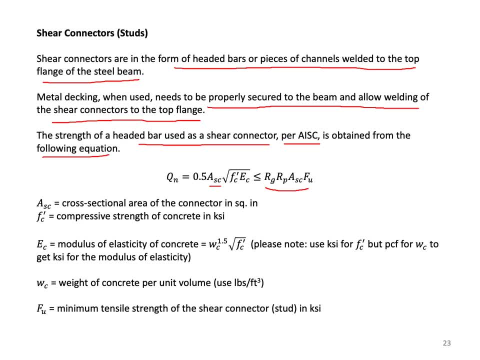 that's 0.2 square inches Your prime sub C compressive strength. but we use KSI for concrete EC modulus of elasticity of concrete, which is WC to the power of 1.5 square root of prime sub C. 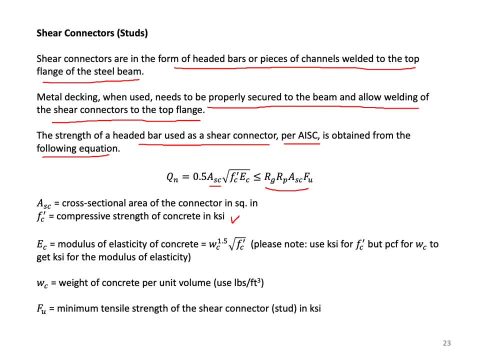 Now, what is this WC? WC is the density of concrete. We use pounds per cubic foot for it. However, for the prime sub C in this equation, we use KSI. The result is in KSI. And what is WC for normal weight concrete? 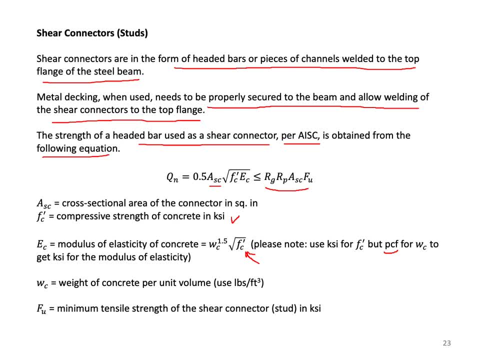 It's about 150 pounds per cubic foot For lightweight concrete anywhere from 90, maybe 100, 110.. And Fu is the minimum tensile strength of the shear connector And usually the value is around 60 KSI, 58 or 60 KSI. 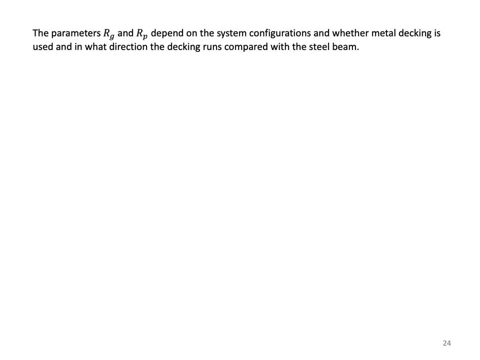 Now, what are the parameters? RG and RP? These depend on the system configuration and whether metal decking is used and in what direction the metal decking is used. If no metal decking is used, then the two factors each is equal to one If decking is parallel to the steel beam. 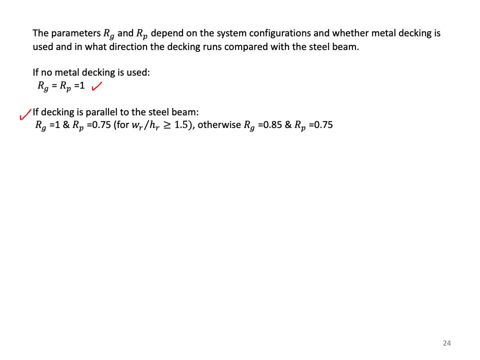 and for the condition the WR over HR is larger than one and a half. Let me show you again what WR and HR are. In that case, RG is one, RP is 0.75.. Otherwise it would be 0.85 and 0.75,. 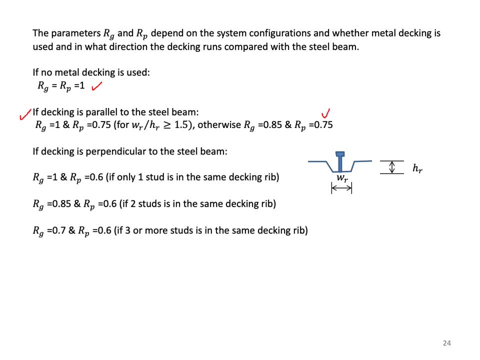 as you can see listed here. Now, if decking is perpendicular to the steel beam- which is, by the way, preferred by many designers, because when the metal decking is perpendicular to the beam, AISC of course requires securing the metal decking to the beam. 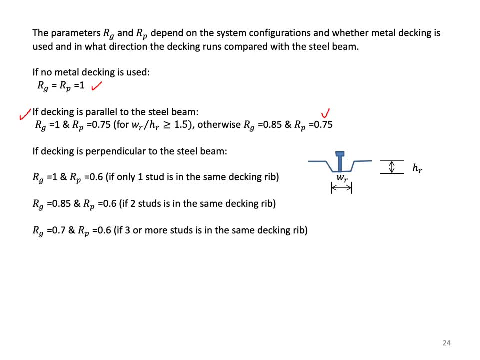 But when it is perpendicular it provides a lateral support for the beam. So during construction you have almost full lateral support. If you're using parallel to the beam, you cannot rely on the decking as a lateral support. I'll talk about that in an example. 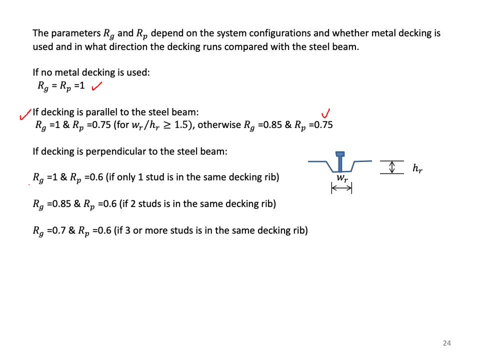 If you're just using one stud per rib, then these are the factors one and 0.6.. If you're using double, like twin, two together, these are the factors, And if you're using three or more, which is pretty rare. 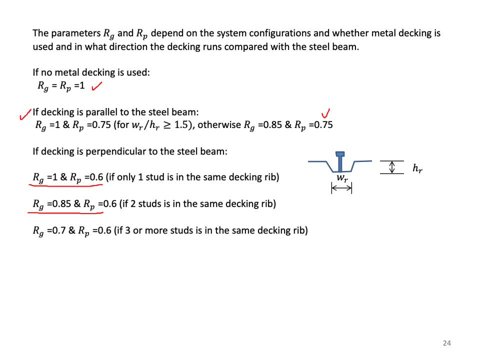 you're using these factors, And usually it's either one or two. Okay, There are variations from these. Sometimes AISC allows larger than these values, depending on certain conditions, so consult with AISC The equation that I gave you, by the way. 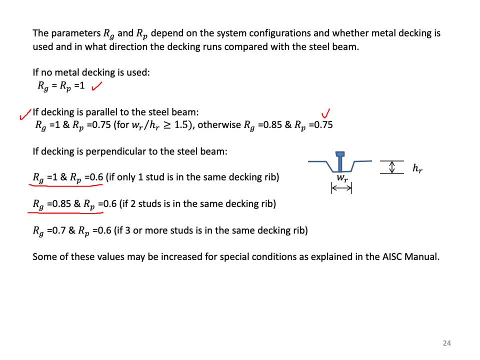 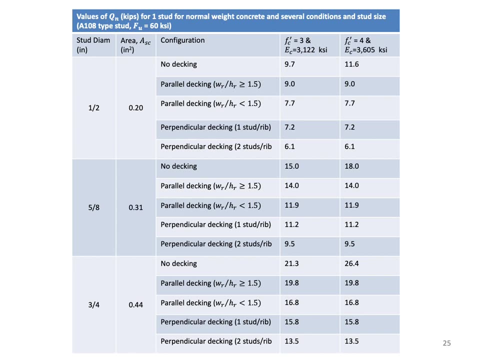 is for metal studs. bars Like bars. if you're using channels, you use different equations. Please look at AISC for equations. when channels are used as connectors, All right, What I did for normal-weight concrete and using AISC, I used CM108 for these studs. 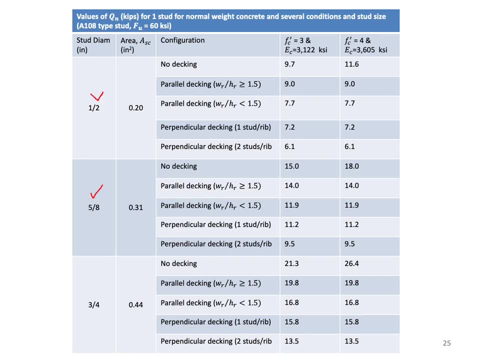 And for different diameters, for three kinds of diameters, and these are pretty much the three that we can use. I computed the values of QN for 3-KSI concrete and 4-KSI concrete, But please notice that to certain points 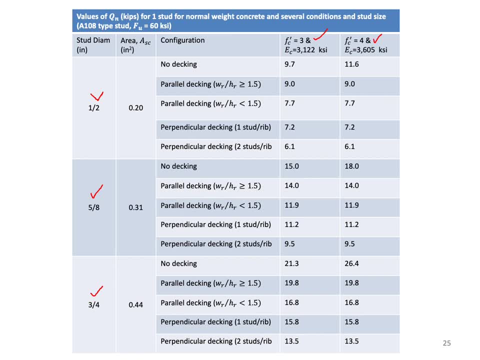 the type of concrete really doesn't matter anymore. Look at here, for example. These values are pretty much the same, So it's more the material of the stud itself that contributes to the strength. Also, notice that, for example, when we are using the metal decking perpendicular. 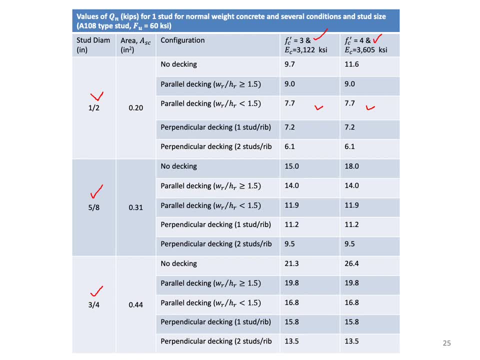 to the direction of the beam. if there is one stud per rib, the value is 11.2.. If you use two studs, it's 9.5.. Now, it doesn't mean it is small Here the stud. 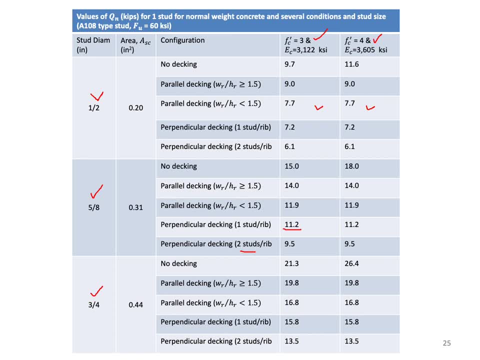 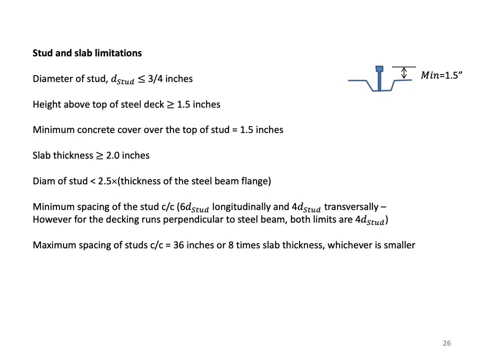 And remember there are two studs. So 2 times 9.5 you use in your equation. So this is a handy table. We're going to come back to this when we are going to do design for the connectors. There are certain requirements for the studs. 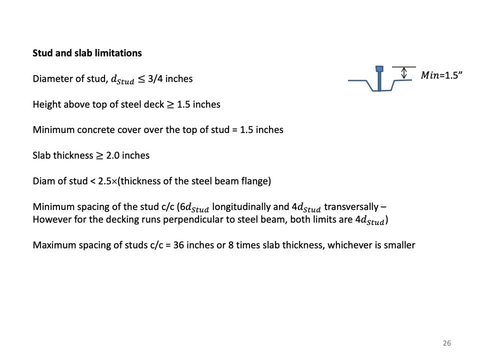 and the slab thickness. The diameter of the stud is limited to three-quarters of an inch or smaller Height above the top, as you can see in here, the top of the corrugated or metal stud, if you have one, at least one-and-a-half inches. 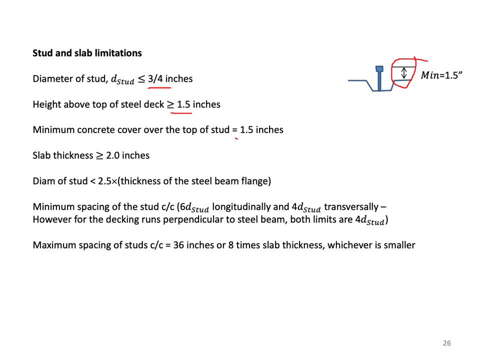 The studs, of course, are buried in concrete, but you need to have one-and-a-half inches minimum protection cover at the top concrete cover. that is The slab thickness. smallest value possible is two inches. The diameter of the stud has to be. 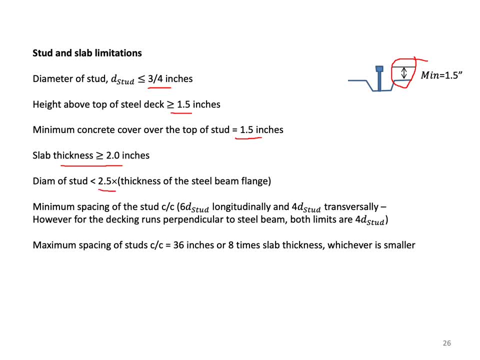 less than two-and-a-half times the thickness of the top flange of the beam. Minimum spacing of the stud center-to-center, six times diameter of the stud longitudinal, four times diameter of the stud transversal, If you are using decks. 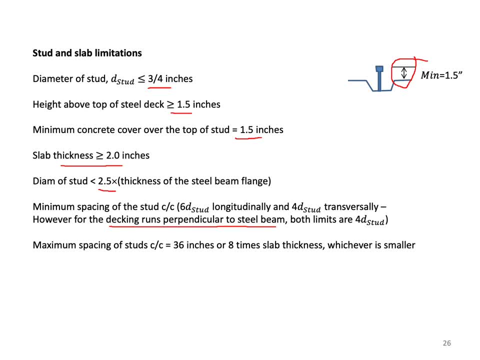 that are run perpendicular to the beam, then both limits are four times diameter of the stud. That's the absolute smallest possible space you can have. Maximum spacing center-to-center is 36 inches or eight times the slab thickness, whichever is smaller. 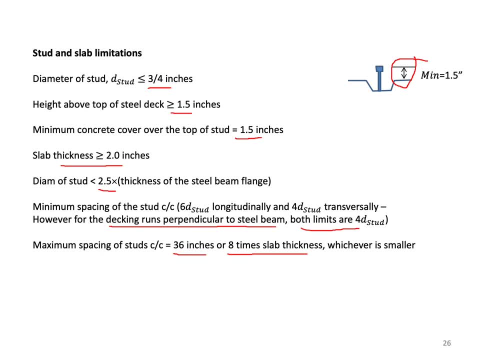 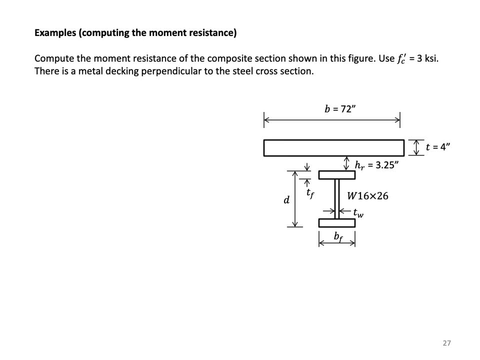 So these are the limitations and make sure that when you design, follow those. All right, let's look at some examples. We want to find the moment capacity of these systems. The thickness, four inches. concrete type 3 KSI. 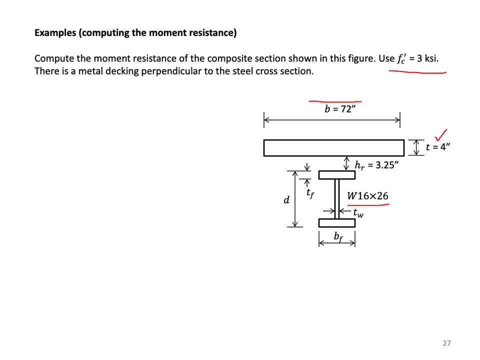 effective width is 72, is a W16 by 26.. We have metal decking which has a height of 3.25.. By the way, the minimum metal decking height is three inches, so we are almost like the minimum in this case. 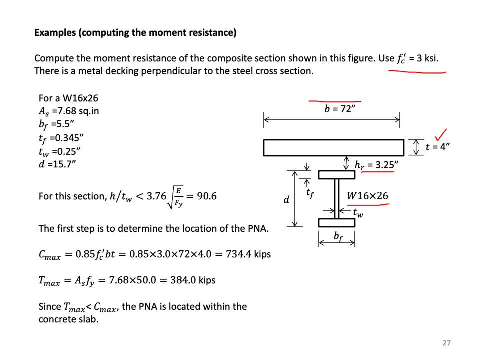 So we go to AIAC table and get the properties of this section. These are the values we need to use, so make sure to list them all And we don't have to check this, but nevertheless I did it. H over TW. 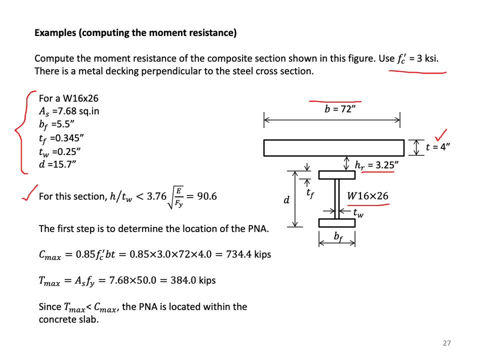 I got the H from the AIAC table And it is smaller than this limit. Okay, the first step is to determine the location of P and A. For that you need Cmax, you need Tmax. I used the equations that I gave you before. 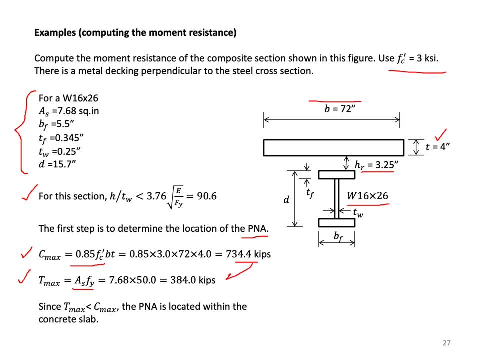 As you can see, here we are talking about a larger value than that one. So what's the condition? That's when P and A is located within the concrete slab. This is usually the case for most floor systems. The location of the P and A. 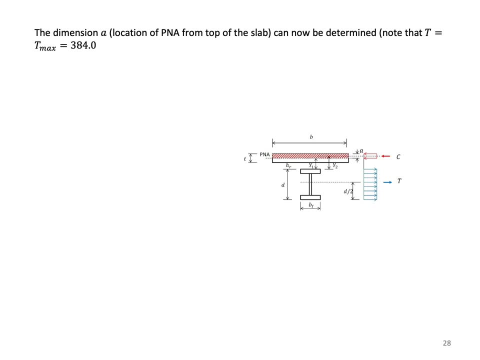 I put my figure back again so we can make a reference to it is distance A. So notice that the T, the tension force, is actually the same as Tmax in this case. Therefore, we use our equation for A and you get 2.09 inches. 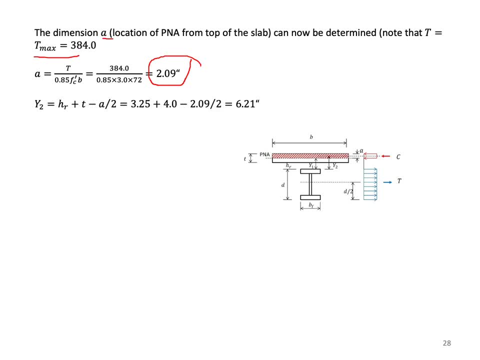 That's A Remember. the thickness is 4 inches, So you get Y2, and that's it. You get Mn T times D over 2 plus Y2, and you're talking about 5,399 inch-kips or 449.9 foot-kips. 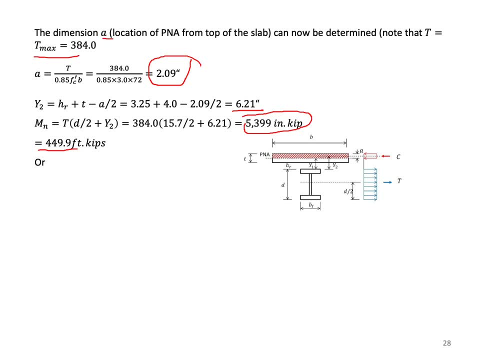 And if you have 5 Bmn, just multiply by 0.9.. Alright, so I did it. So that is the factored resistance, Alright. so what is the horizontal shear In this case? sigma Qn is Asfi. 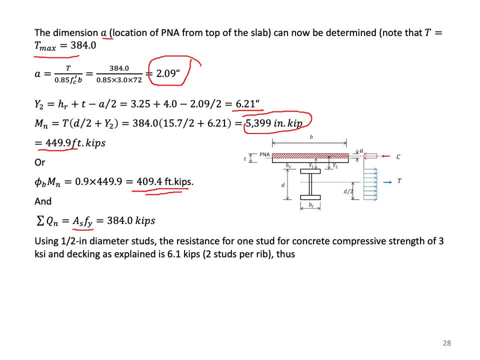 Let's design for connectors, So let's use a 1⁄2-inch diameter stud. Go over the table. The resistance for one stud when the 3 KSI concrete is used is 6.1.. And if I use two studs per rib, 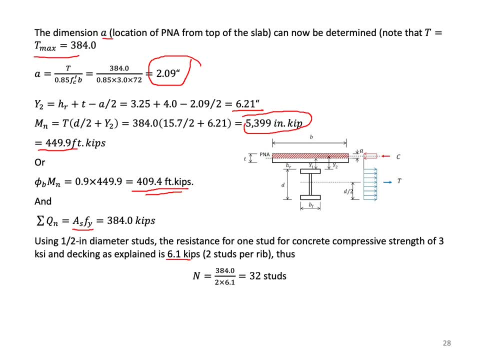 it's 6.1.. Alright, so you get two studs per rib And therefore N. the total number of studs needed is that horizontal shear multiplied by 2 times the strength of 1, and you get 32 studs. 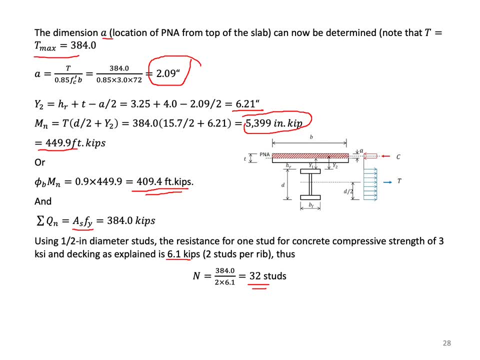 So this is if it is a simply supported beam, this is over half of the span, Right? So one half of the span requires 32.. Totally, 64 studs would be needed. You can figure out what is the spacing by knowing the length of the beam. 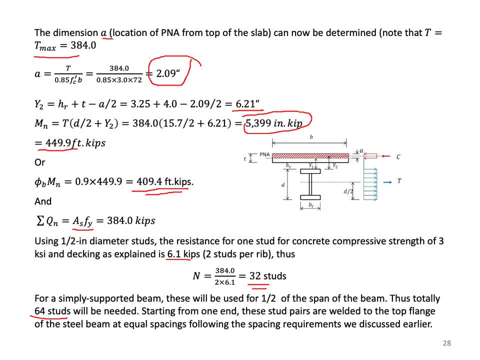 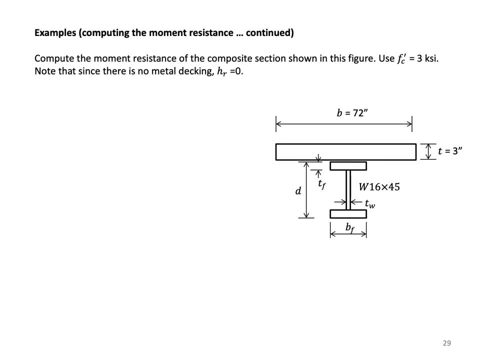 The problem didn't give us the length. so if you have the length, you compute what the spacing is and check the spacing with the requirements of the AISC. Alright, let's look at another example. In this case we don't have any metal decking. 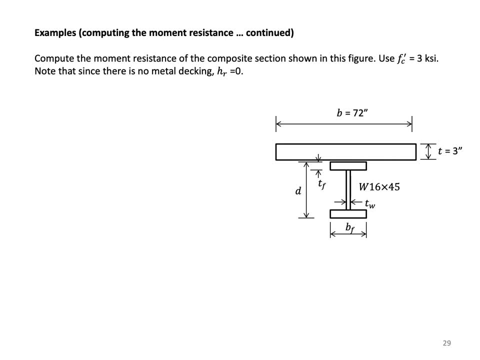 The thickness of this slab is 3 inches And we have a W16 by 45.. The effective width is 72.. The HR is equal to 0.. So I again went to AISC and listed the properties of this section. This is satisfied. 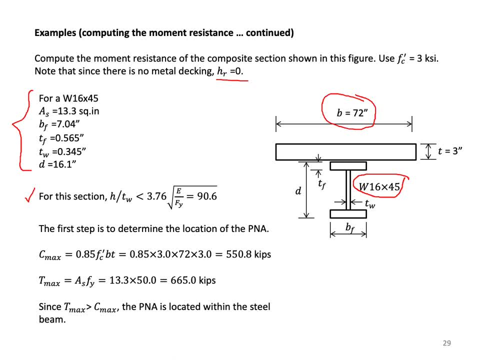 I don't have to check it, but I, just as a habit. I always do it. And then the first step is to determine the location of PNA. I computed Cmax and computed Tmax And look at here, This is now larger. 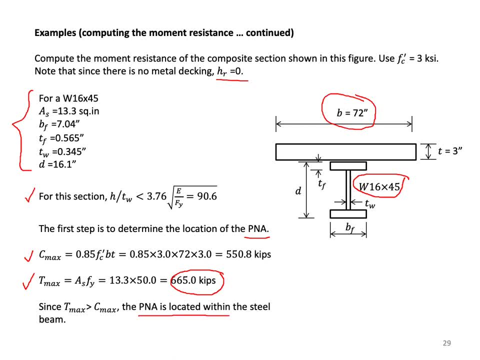 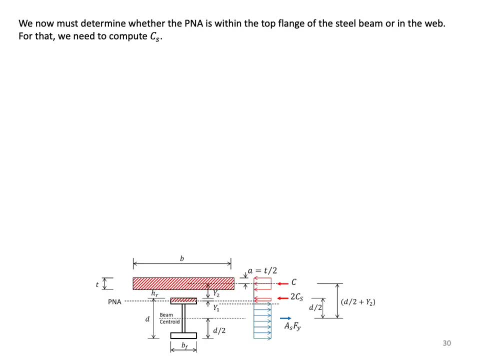 What does it mean? Well, that means PNA is located within this steel, So let's see how we can continue. I put the diagram back when the PNA is within the steel, but we don't know whether it is in the top flange. 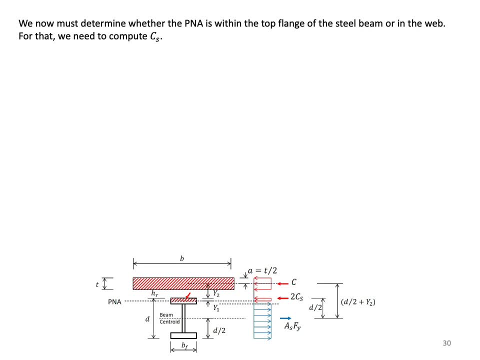 or it is in the web, But let's say that this is the situation. So let's find CS first. Remember it's ASFI minus C, divided by 2. So we get 57.1.. And the C flange. 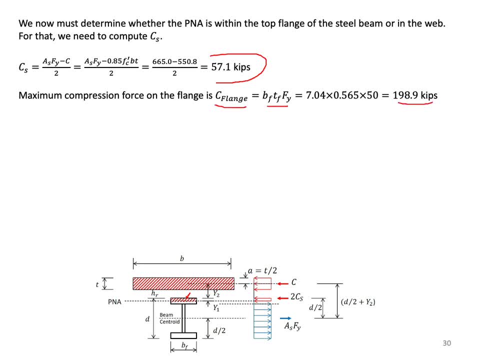 the maximum compression of the flange is 198.9.. So what does it mean? This is smaller. So that means it is just like the figure that I have shown in here. It is in the top flange. So what do I do next? 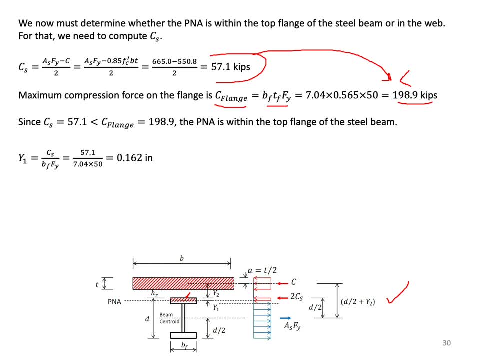 Well, find out what is Y1 by dividing CS by BFFY. So it is really extended a very small amount into the flange. It's just about 0.162 inches below the top flange, So I compute the Y2. 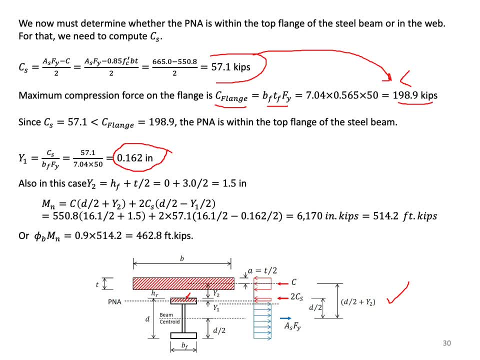 as I gave you before. I put it in the equation for MN, and after multiplying by the reduction factor, I get 462.8 foot kips as a capacity in this case. Alright, so the next question is: what is the horizontal shear? 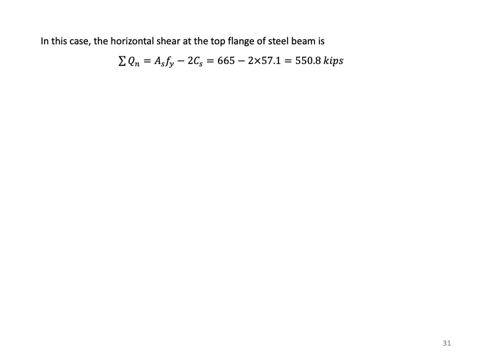 I gave you the equation ASFI minus 2C sub C 550.8. and let's say, if I use now 3 quarters of an inch diameter stud for a prime sub C, going over the table, I get 21.3.. 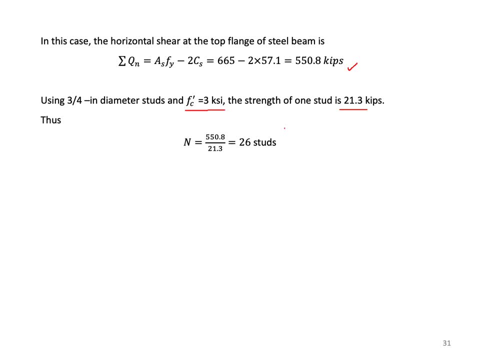 Just one stud per rib And that gives me 26 studs. totally needed. Again, if it is simply supported, beam over one half of the length of the beam. If it is not simply supported, you might say is over, what length Is over? remember? 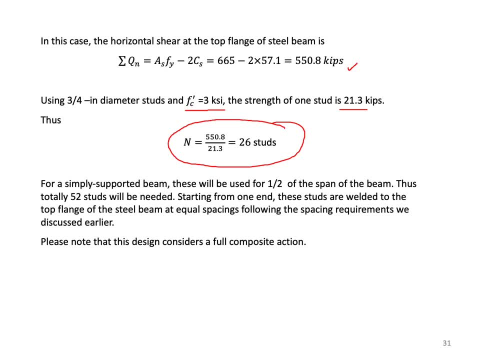 point that bending moment is 0 to where bending moment becomes maximum. So, totally, we need 52 studs. Again, find the spacing. check AIAC, those limits that I gave. make sure that you are following the requirements. Alright, Now what is the design procedure? 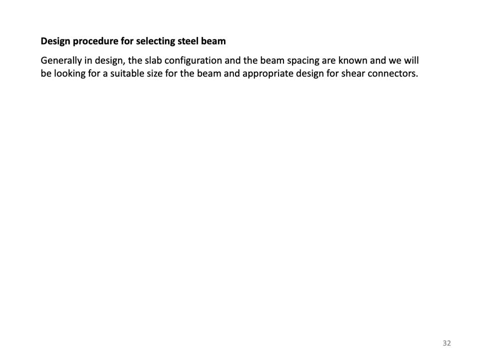 when we don't know what steel beam we have. In that case, generally the slab configuration and the beam spacing are known. So we have that from architectural drawings, from experience, and therefore the parameters that are known, we can determine. 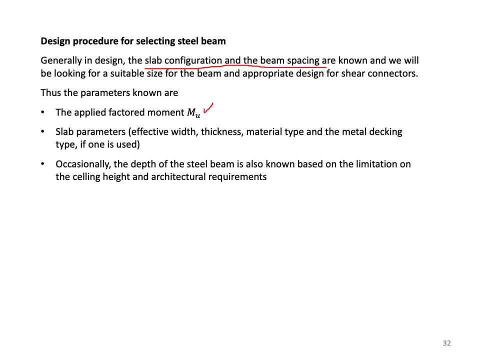 one is MU. You might say: I don't have the weight of the beam. how do I compute MU? Just assume a value, maybe 60 pounds per linear foot, 70 pounds per linear foot, and continue with the calculations. We have this slab parameter. 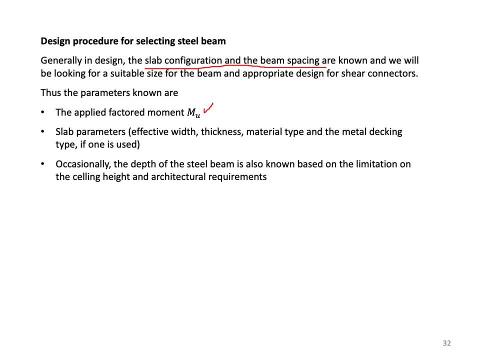 we know the thickness usually, we know what kind of slab, we know whether there is a metal leaking or not, And listen to this. occasionally we even know the depth of the steel beam. We don't know what size, but some architectural drawings. 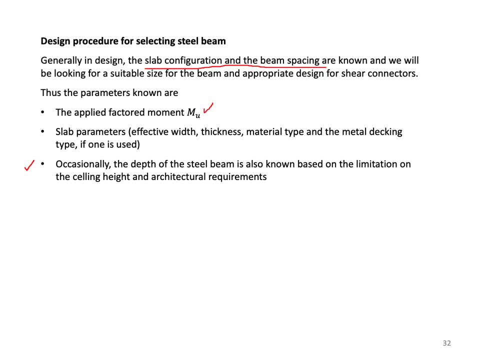 and limitations of the ceiling tell us that this should be the depth of the beam, So sometimes you even know that. So if these are the case, I've introduced two different methods. One is called the conservative design And it's based on the condition. 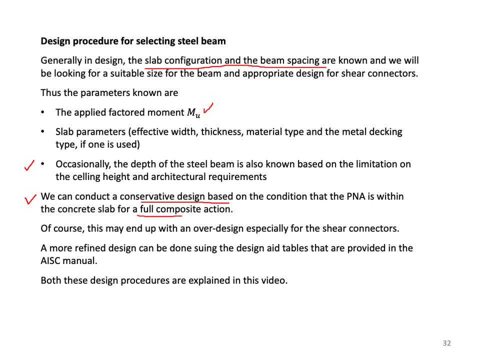 that PNA is within the concrete slab for a full composite action. This may end up with an over design, especially for the shear connectors, And you use the maximum number of shear connectors to get the full composite action. A more refined method is in AISC. 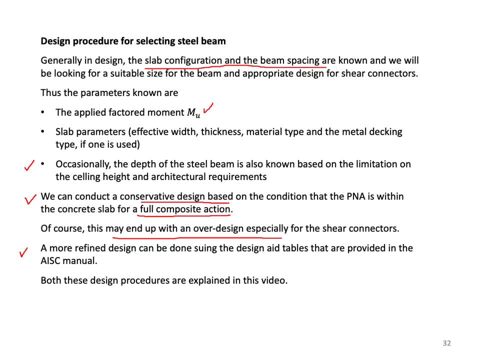 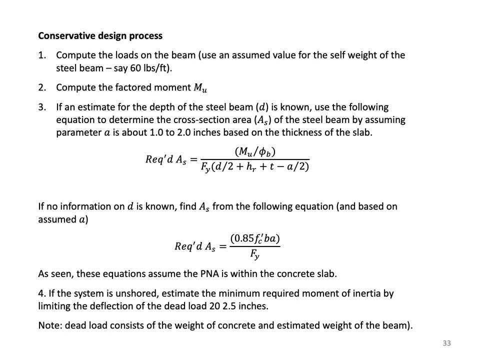 using tables. That would give a less conservative design and a design that is more comparable with the amount of moment that you have applied on the beam. So in this video I'm talking about both these methods. Let's look at the conservative design process. 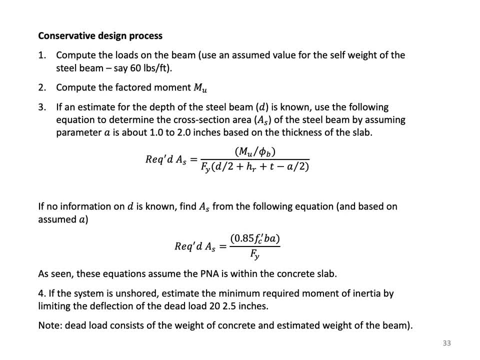 You can use this without a need to go over the design aids. So you compute the loads on the beam and assume the value- as I said, the self-weight of the steel beam, Then compute MU with load factors If you know what depth you have. 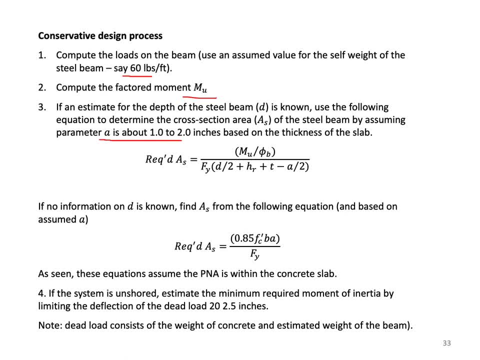 for your beam. assume A is equal to maybe one or maybe two inches, depending on the thickness. Usually I use two inches And find out what is the required area of the steel. So what I'm doing, just using the moment. 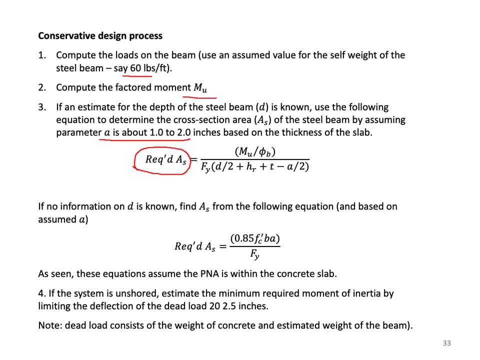 you notice that I am dividing the MN by phi, because this is the required value, for actually this is MU, MU divided by phi. This is the required strength, without the reduction factor, And then I'll simply dividing this by the lever arm, because A is already assumed. 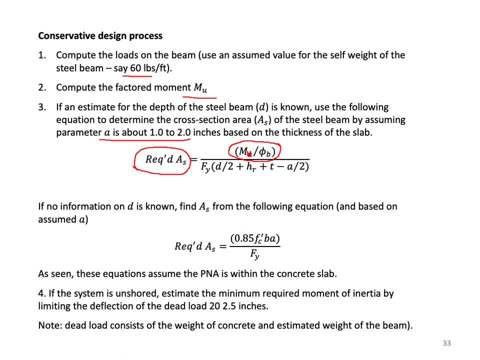 Assuming that the PNA is within the top flange, as you recall. If you don't have any value for the depth of the beam and you really have no clue what the depth should be and have no experience, then simply use this equation. 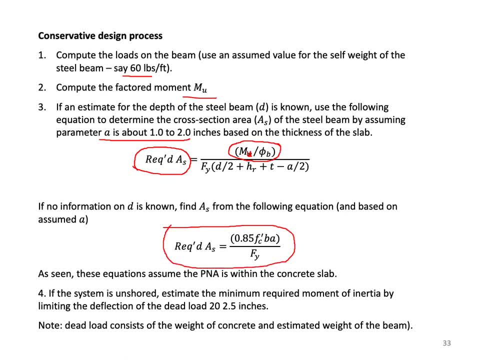 This is based on the equilibrium of the forces- Compression force divided by tension- and you solve it for AS. So now we know what area we need for our beam. So again, notice that the PNA is between the concrete slab, If the system is unsure. 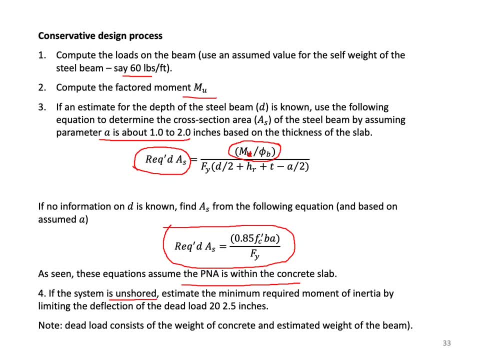 now- this is important- estimate the minimum required moment of inertia by limiting the deflection of the dead load only to 2.5 inches. Dead load consists of the weight of the concrete and estimated weight of the beam. Alright, So how do I do that? 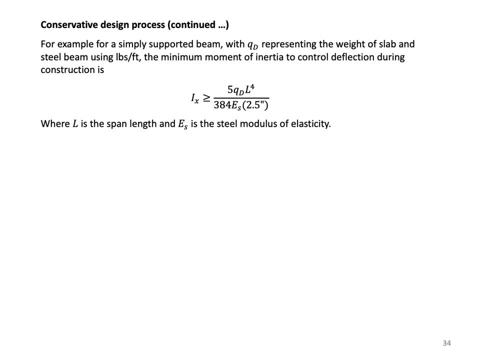 If it is a simply supported beam, you know the equation for deflection and solve the equation for moment of inertia for 2.5 inches. maximum deflection during construction. ES is the modulus of elasticity of the steel and L is the length of the beam. 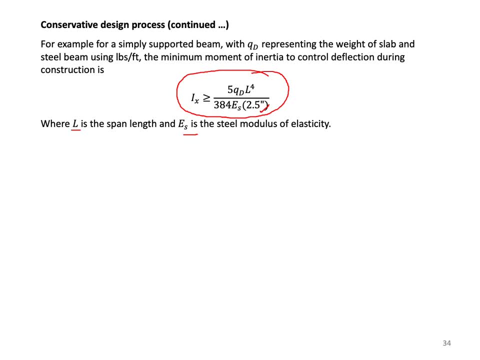 And make sure that you use inches and pounds in the entire equation, including the load QD. Usually it is pounds per foot, so divided by 12. 12 pounds per inch, And then select a suitable section and compute the bending resistance: phi MN. 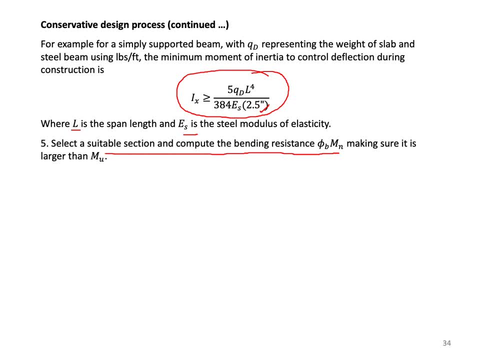 Make sure it is larger than MU. So that is pretty simple. Decide on the connector diameter and determine the number of shear connectors using the equation that we used before. If it is an unsure system, make sure the steel beam alone is able to sustain. 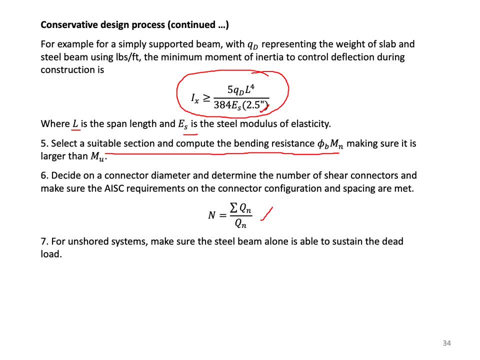 the dead load, And not only you check the deflection of it during construction. make sure that this beam is not composite yet. So is it able to take the dead load? Usually it does, but nevertheless check it, And for all kinds of decking. 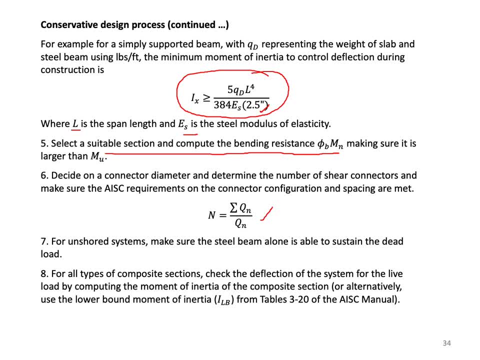 whether there is a decking or no decking. you need to check the deflection for the live load to make sure that it is less than L over 360, as I talked about, And for that the easiest way is to either compute the moment of inertia, 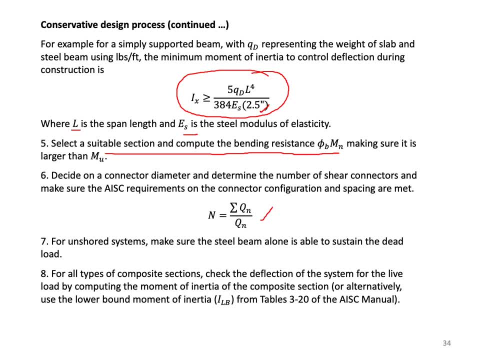 based on the what we call transform section or, more conveniently, use a value called ILB. LB means lower bound. There are a series of tables- maybe two tables, I think, or maybe three- in AIAC called Table 3-20.. 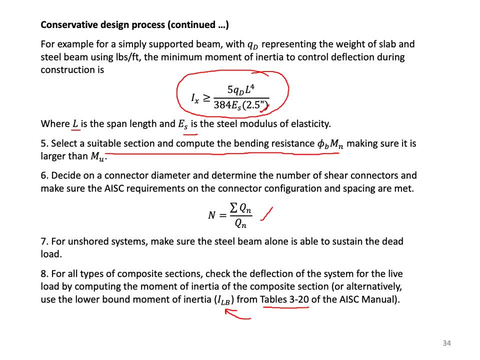 And this value is listed for different sections. You can use this value for computing deflection. Finally, make sure to check the shear. As I said, we don't talk about shear except for design of connectors. but this is the shear on the beam. 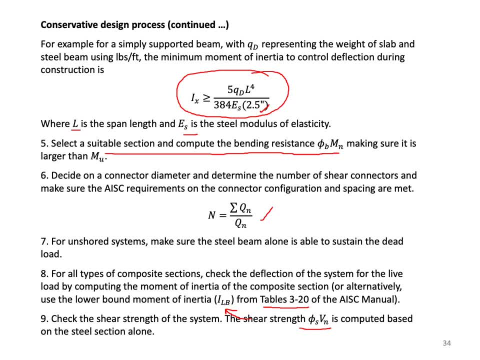 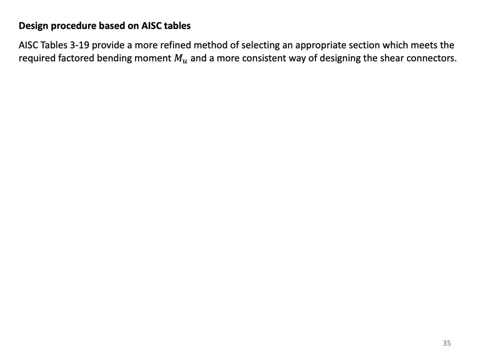 When you check the shear, there is no composite action. It's just the steel beam alone that must take care of shear. So that's pretty straightforward. All right. Now let's talk about design based on the AIAC tables. These tables are designated. 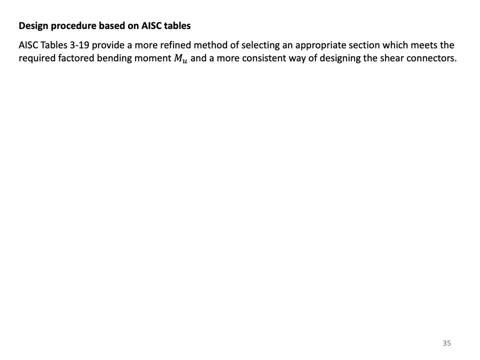 as Tables 3-19 in AIAC, Very useful tool for designing the composite sections. For that, of course, you always need MU And again: assume a value of the self-weight of the beam. Assume an initial value for parameter A. 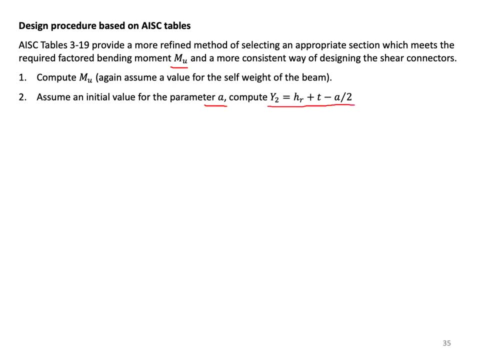 and compute Y2.. All right Now, because in the limit we have the reduced capacity the same as MU, so we can use MU in our equations. The AIAC tables list the phi BMN based on the two parameters Y2 and seven different levels. 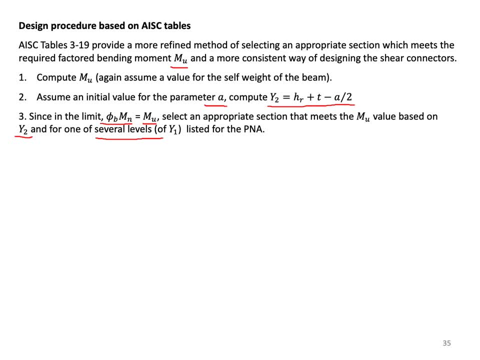 of parameters Y1. There are seven different levels of P and A. So these seven different values, two are for the P and A locations at the top and bottom of the flange of the steel beam, three within the flange and two below the flange. 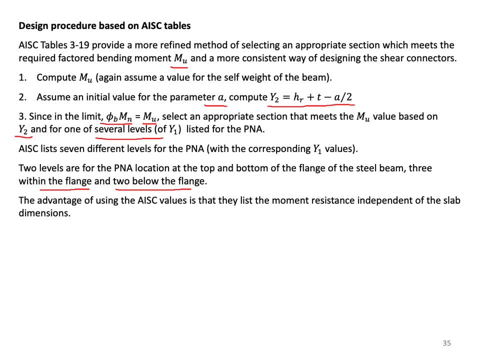 The advantage of using AIAC values is that they list the moment resistance independent of the slab dimensions. All you need is the slab thickness, You don't need to have B. So that's the good thing about the AIAC tables. However, 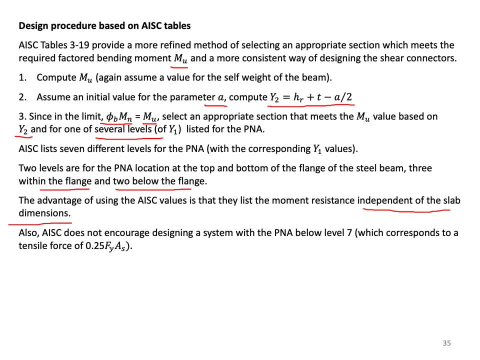 AIAC doesn't encourage designing a system with the P and A below the level seven. That is corresponding to a tensile force of about 25% of FYAS. All right, So with the section that you select from the table, and I show you how it is done. 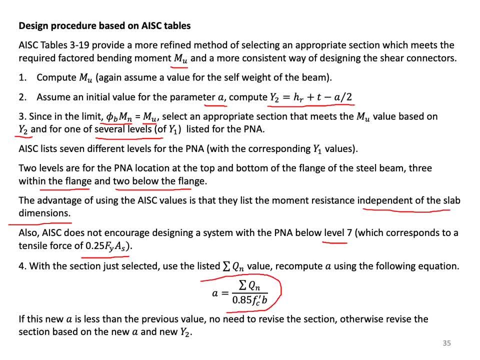 you compute A, which is this equation. You might say: well, you never had A equal to this. But remember that sigma Qn is the same as a tension force, So it's a tension divided by pretty much the value. 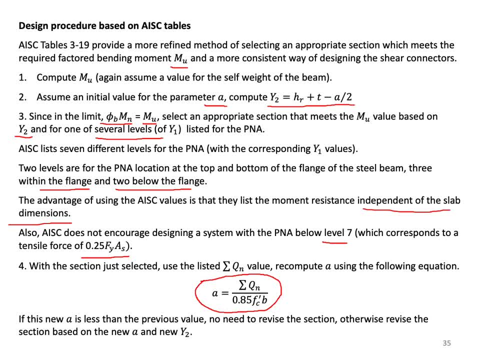 the concrete value, In other words tension equal to compression, And from there you compute A. If this A that you find is less than the one you assume, that is it. You don't have to repeat any calculations. If it is larger than the A. 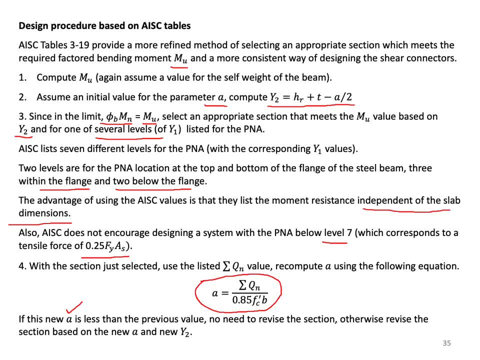 that you assume. that means you are, you know, outside, maybe outside of the concrete or the value you know. the compression force now is a little bit larger, so you have to go back and revise your calculations, Probably pick up a larger section. 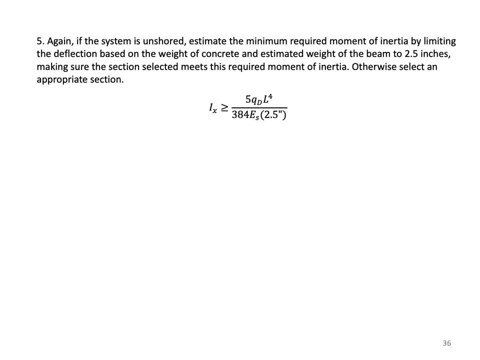 All right. And again, if it is a situation that you have no sure use in your design. so during construction you want to make sure that deflection is not large, so the section you select must have a moment of inertia at least equal to this value. 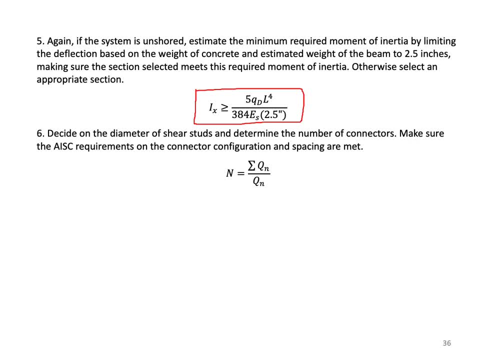 And the rest of the process is as before. You have sigma Qn, which is also listed in the table, divided by the strength of one connector, and you design the number of connectors And and also as a check during construction. 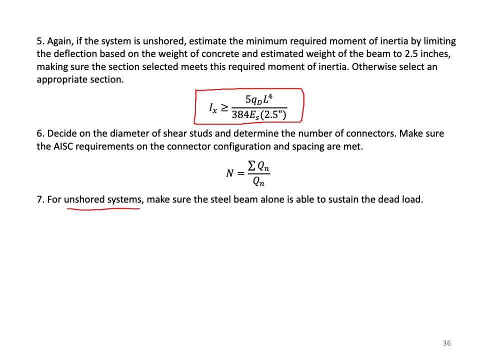 if it is on short system, make sure that the steel itself has enough strength bending resistance to carry the bending moment applied because of the dead load- And that's a very easy step- And regardless of the type of the composite section, whether short. 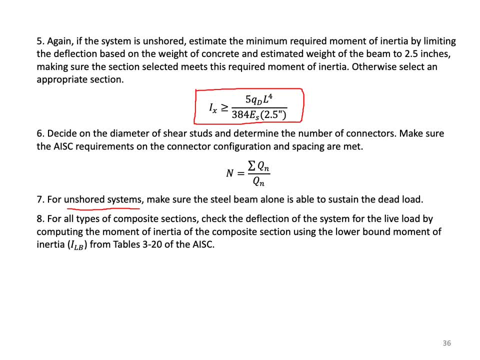 unsure, whether with metal decking or not. always check the deflection after the composite action is done, And for that you can use the ILB that I talked about from tables 3-20 of AIAC. Make sure that deflection for the live load only. 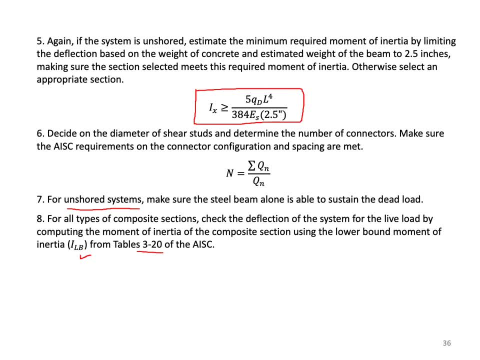 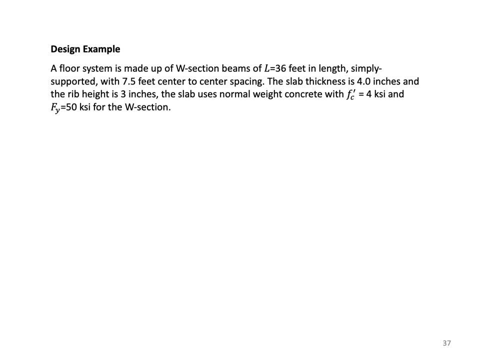 is less than L over 360.. Okay, And don't forget to check this year, as we talked before. So let's look at the design example. We are talking about the W section used. The span is 36 feet simply supported. 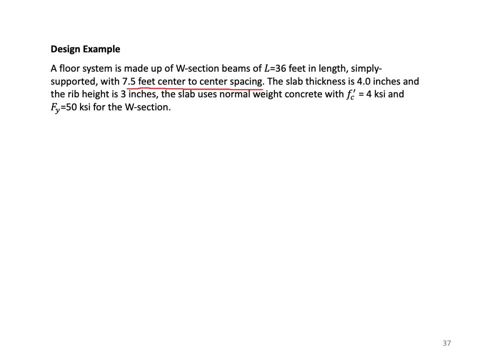 7.5 feet center to center spacing. The slab thickness is 4 inches, The rip height 3 inches. The slab uses normal weight concrete prime cell C4, KSI, FY50 for W sections. Metal decking is perpendicular to the steel section. 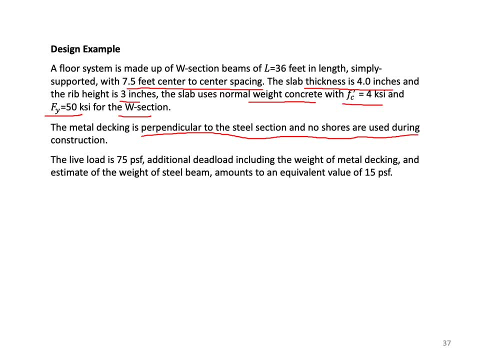 and no shores are used during construction. Live load: 75 PSF. Of course, the dead load is because of the slab, but there is an additional dead load of 15 PSF using for the metal decking and converting the estimated weight of the beam. 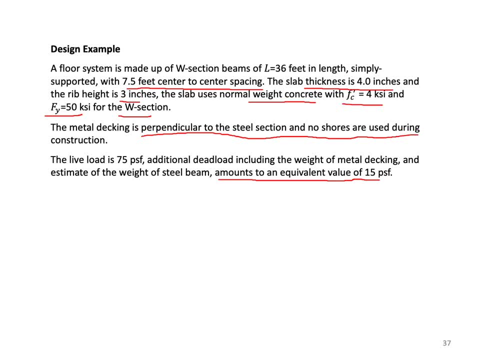 as a floor load, so that's about 15 PSF. All right, So let's do it for a typical interior beam. Remember the equivalent B, rather effective B. that becomes 7.5 feet, so it's 90 inches. 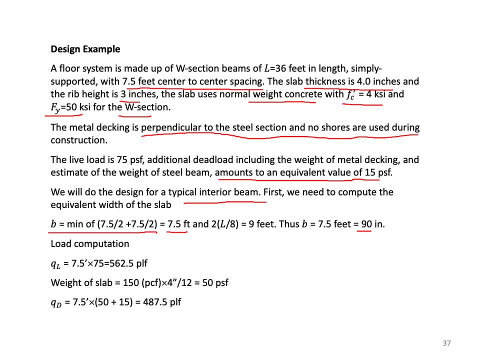 We compute the loads. for the live load, the tributary width is 7.5, so we get 562.5 pounds per linear foot. Weight of the slab is 150 pounds per cubic for normal weight multiplied by the thickness, divided by 12,. 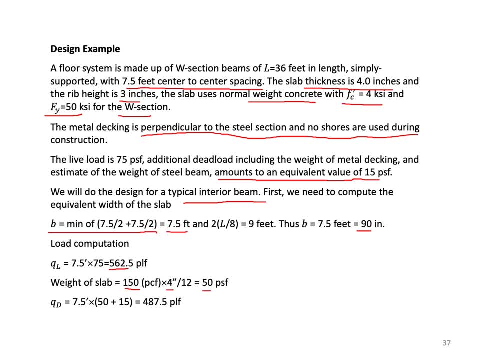 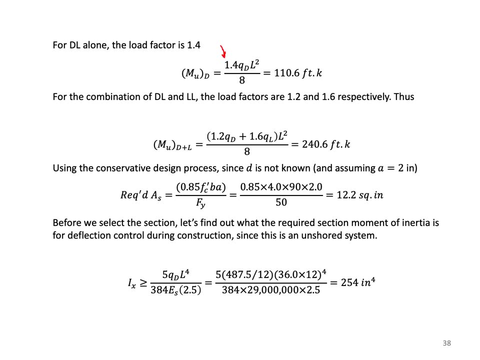 so we get 50 pounds per square foot. I add to that the additional dead load multiplied by tributary width and I get the total dead load All right. So if I use the dead load alone, with the load factor of 1.4,. 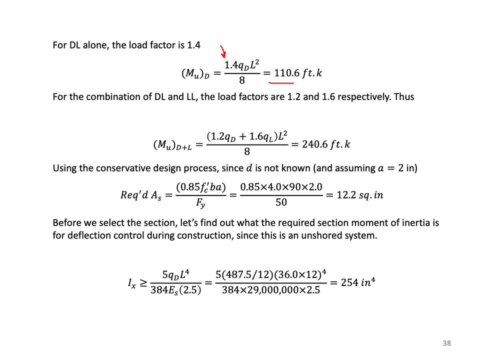 I get this amount of moment. If I use a combination of dead load and live load, I get this moment. This is during construction, this is after All right. So let's say, I don't know what the D is, so I use the second equation. 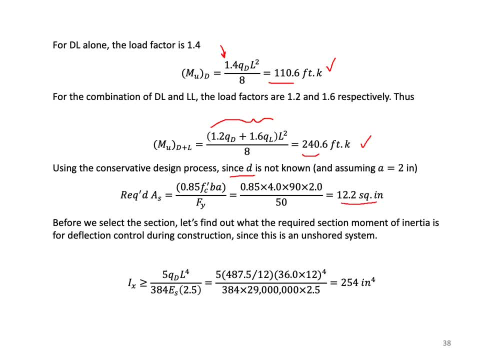 I gave you, and that is roughly the area I need. You don't have to really stick with this. You can go a little bit lower, and actually that's what I'm going to do in this case. So, but before I do that, 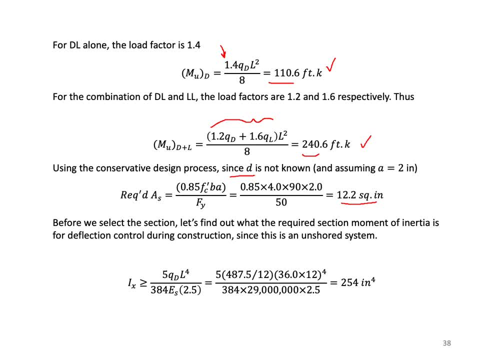 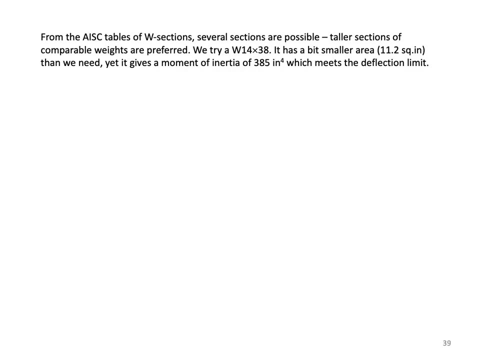 I also check with the construction, the deflection during construction, and I realize that I need 254 inches to the third as a moment of inertia. So when I pick up my section I keep this number in mind. All right, So I can try a W14 by 38.. 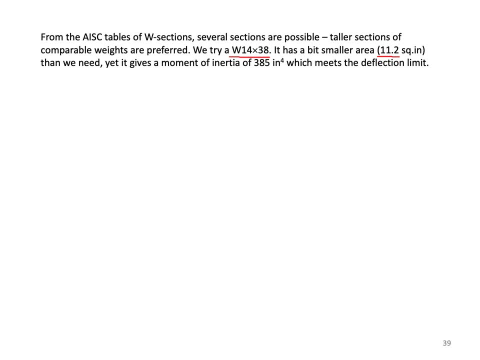 It has a W14 as an area, a little bit less than what I need, but it has a moment of inertia. So since metal decking is perpendicular to the beam and properly secured to the top flange, the beam is considered adequately supported laterally. 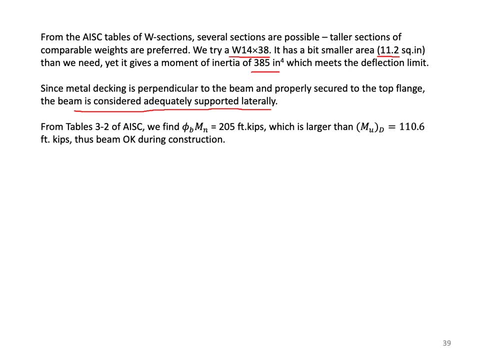 during construction, And table 3-2 of AISC gives me the bending resistance of the beam without the composite action, and so that's larger than the value during construction. so I'm okay. Now here is a very important note. I think I talked about it. 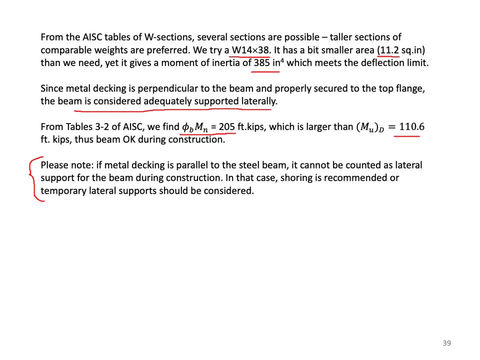 If the decking is parallel to the steel beam, you cannot use the decking as a lateral support. It's ineffective. In that case, you need to have some temporary lateral supports, or definitely you have to have a short system. All right, So let's figure out. 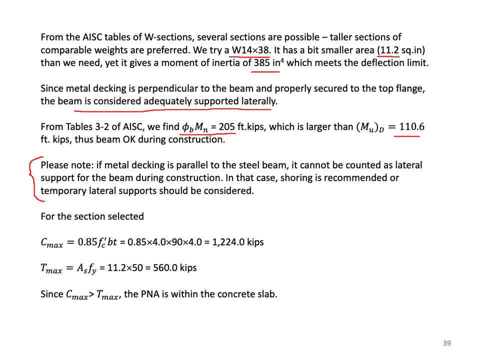 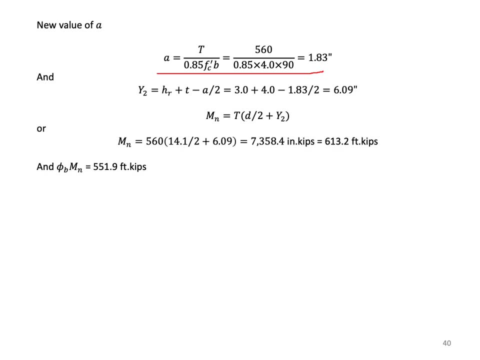 what's the situation here? Cmax- I computed. Tmax- I computed, turns out P and A is within the concrete slab because Cmax is larger. And now let's compute the value for A Y2, and using the equation Mn, I get Mn as 613.2 foot kips. 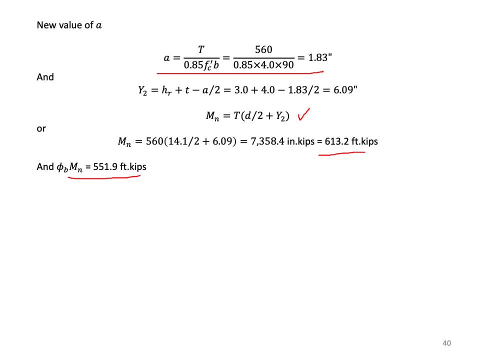 so a large amount of capacity. Now, for this you need to use also the maximum number of connectors, so definitely larger than what we need, And using Sigma Qn, which is AsfY in this case, and I use two studs per rib. 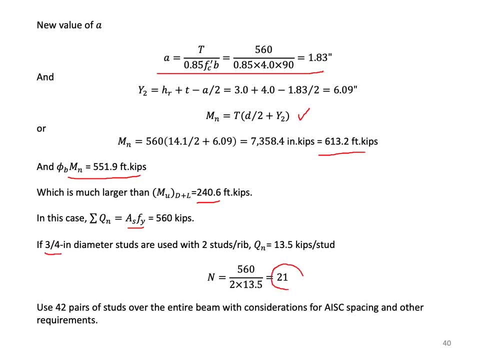 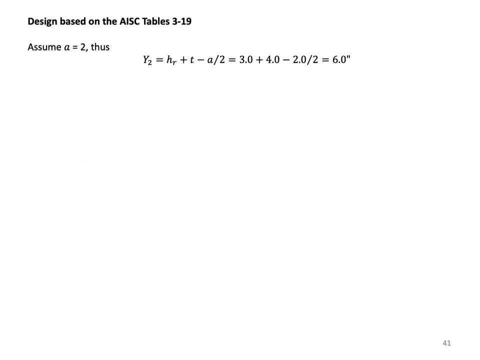 three quarters of an inch diameter. I need to have 21 pairs of studs over half of the length, so 42 pairs total. That gives me full composite action. All right, It's a conservative design. right Now let's look at AIC-based design. 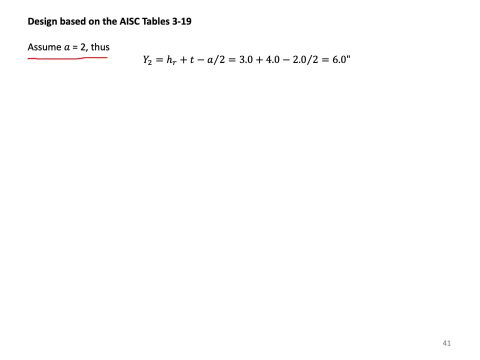 I'm going to assume A equal to 2.. That's where we start And therefore I find Y2, which is 6.. The total moment is 240.6, so I need to find what section has this much of a strength. 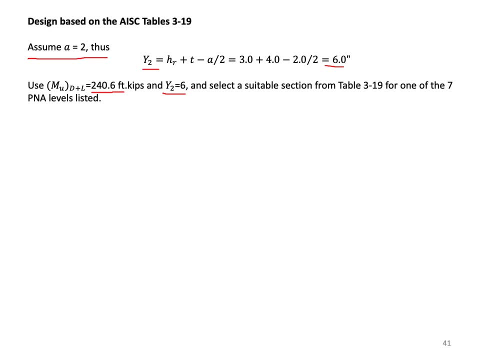 For Y2 equal to 6,. the table is 3-19, and I pick up the appropriate condition for one of the seven P and A that I talked about. I show you the table. momentarily. I saw that there are two possibilities. 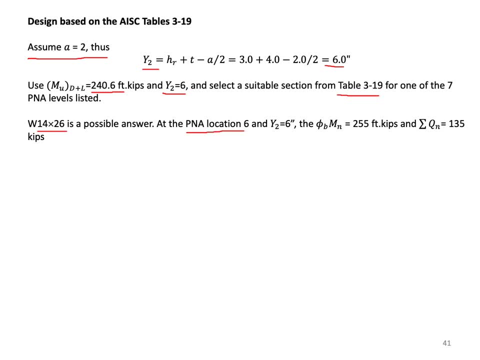 I can use a 14 by 26, P and A location 6, and Y2 is 6.. It gives me this much strength, so I'm okay compared to that one. See that And Sigma Qn listed is 96.. 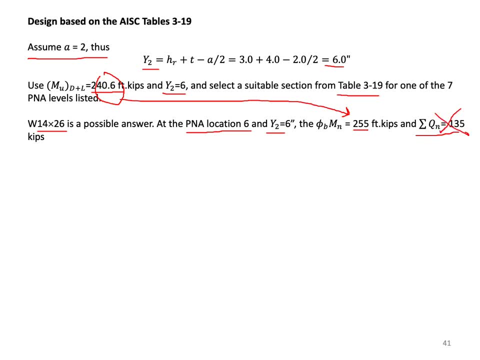 I'm sorry. Sigma Qn is equal to 135 kips, Okay, And the 16 by 26 is another possible answer, but this one is a location P and A location 7, and Sigma Qn is 96.. 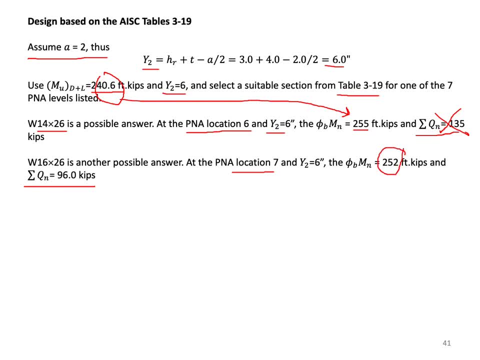 Look at the strength. So we have a good section and you can check either of the two. I'll check this. try this second one and see what happens. I computed A and revised my Y2, and if I use one half an inch diameter start. 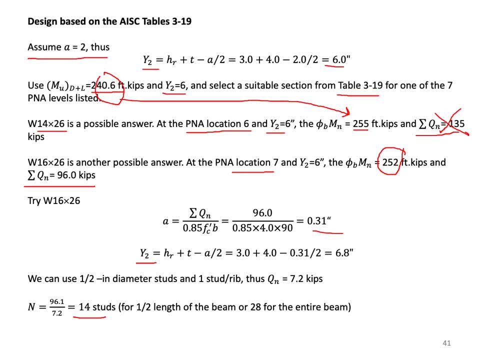 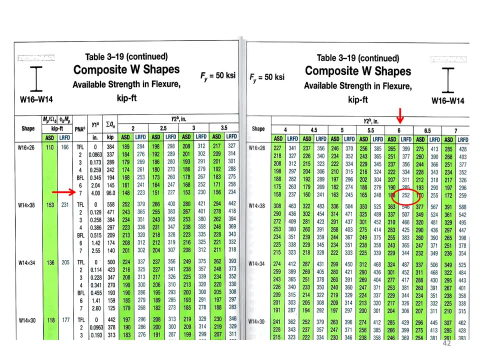 and one start per rib. I only need 14 starts. So this is now not a full composite action. It's partial because the neutral axis is lower, and nevertheless it will provide the strength that you need. So here is a typical AIAC table. 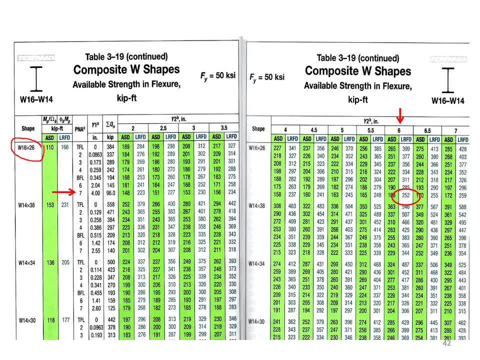 I mark the value that I picked up for W16 by 26.. You notice that P and A locations. there are seven of those. Actually, when you go across- and here is a Y2, you come down for 6 is 252 that I picked up for LRFD. 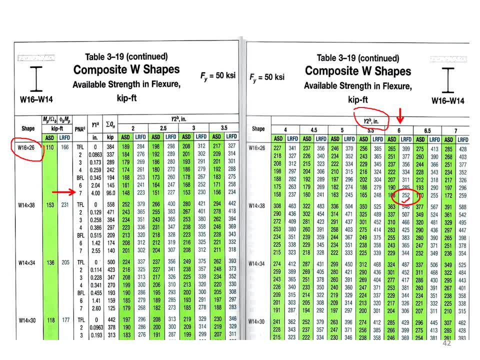 Don't use AST LRFD. And also you notice that the sigma Q is listed as 96.. And for this condition the Y1 is equal to 6.. So it's extended certainly below the slab. So that's how these tables are used. 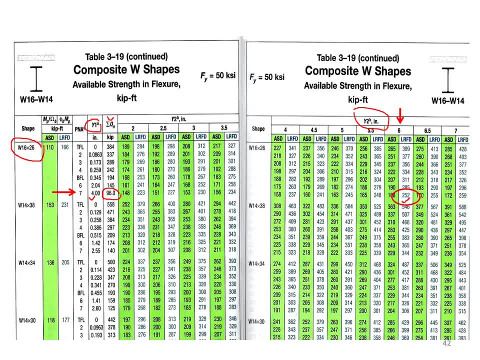 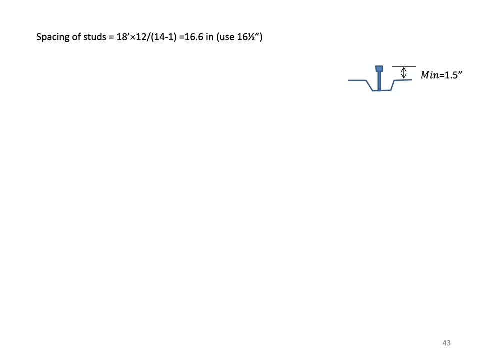 All right, So learn these tables. Let's look at these. starts spacing over the half of the length of the table. So this is the width of the beam. so 18 multiplied by 12, 14 needed, So there are 13 spacings. 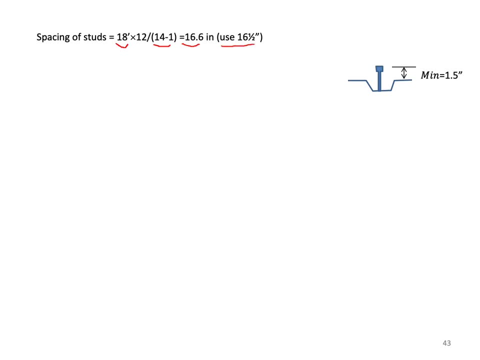 and there is 16.6 inches of spacing. So if I can put like 16 and a half spacing, that should be fine. And minimum spacing is four times diameter, so I'm okay. Maximum spacing is 36, or eight times thickness of the slab. 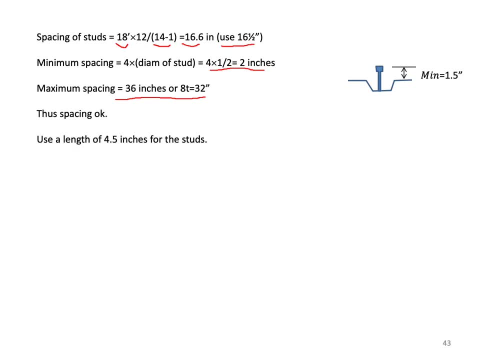 which is 32, so I'm okay. Therefore, the spacing is okay. I need to use at least four and a half inches for the length of the stud because of this minimum that we need. Okay, Let's look at the live load deflection. 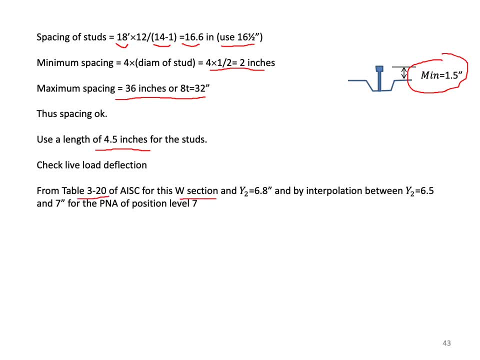 I use table 3-20 of AIC for this W section and because Y2 is equal to 6.8, 6.8 is not listed, but there is 6.5 and 7, so I did an interpolation. 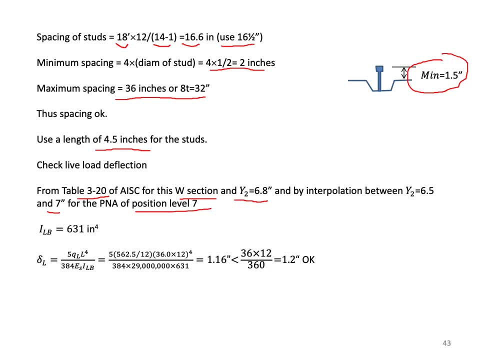 Level is 7.. I show you the table. With interpolation, I get 631 inches to the fourth. so that's the unit for I. I mentioned inches to the three before, but no, the unit for IB is inches to the fourth. 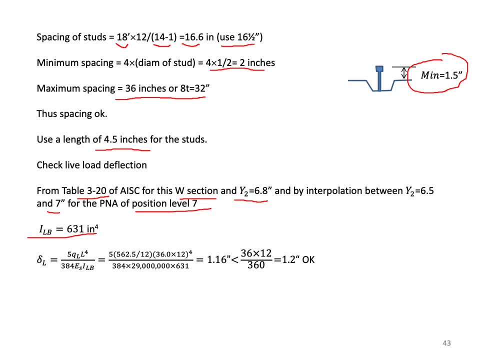 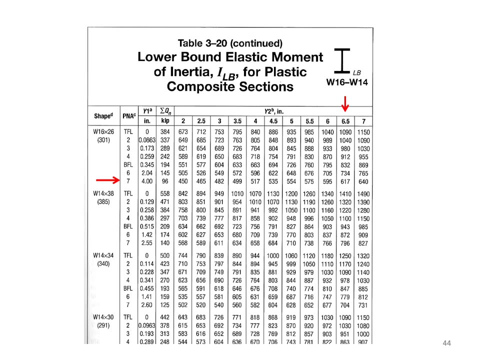 Sorry for that mistake I had earlier, but use the equation for deflection of the live load. Again, use inches and you have to be less than L over 360, so you're okay, And here is a table for what we call. 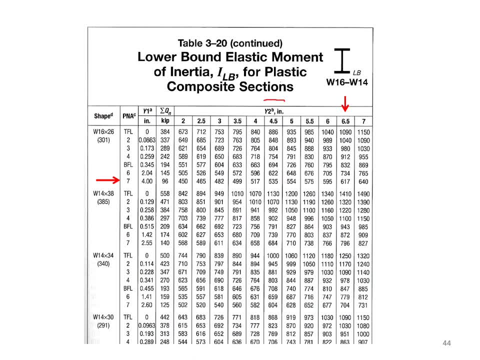 the ILB moment of inertia. You notice that the Y2 is listed for the section that we selected. We are level 7, but we don't have 6.8, so I have these two values: one for 6.5, one for 7.. 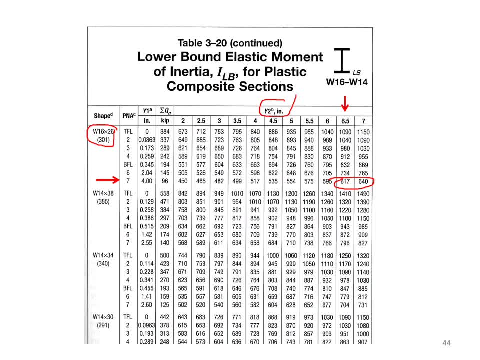 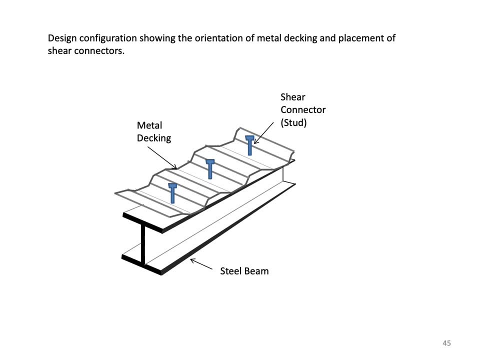 I did the interpolation in between, All right. So I just put this illustration to show you how our design would look like. We got the steel beam, We got the corrugated sheet, We got the studs and our design is completed. 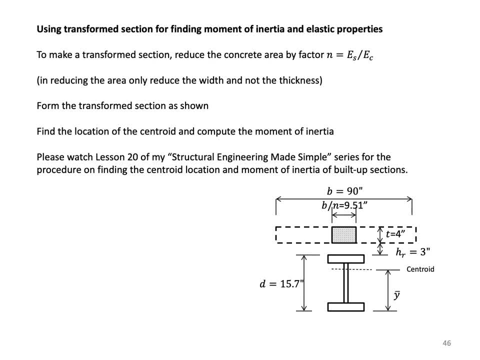 All, right, now the last board. If I want to find the section properties, excuse me- using the transform section. what do I do? Find the ratio of the modulus of elasticity of the steel to concrete. We call it N. Reduce the compression area. 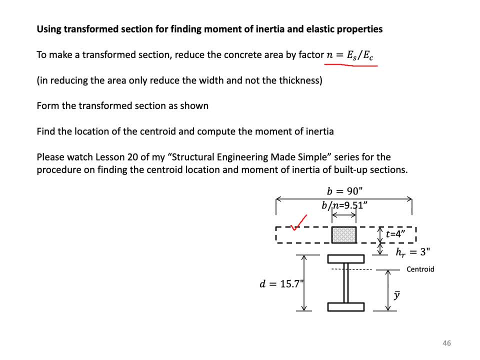 by this factor, by dividing the area by that factor, but we do not touch the thicknesses. We keep the thicknesses as they are: the 4 inches and 3 inches. We only reduce the width. so, from 90 divided by N. 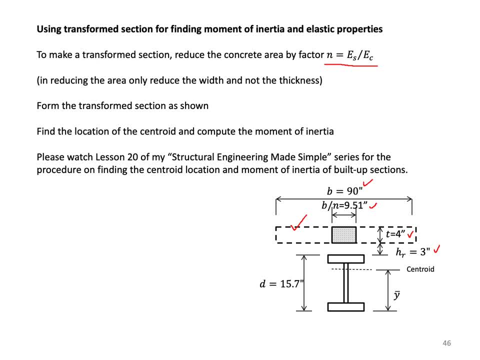 we get 9.51.. All right, And then find the centroid using the equations of statics. Now, if you, if you would like to know how it is done, please watch lesson 20 of my structural engineering made simple. I have a procedure in there. 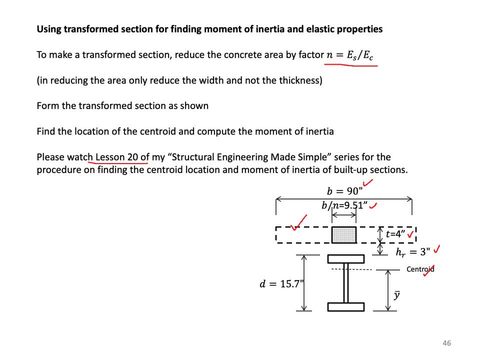 how to find the centroid and moment of inertia section, modulus etc. for any built-up section. So for this one our case N is equal to 9.46, and for W16 by 26,. I need the moment of inertia and area. 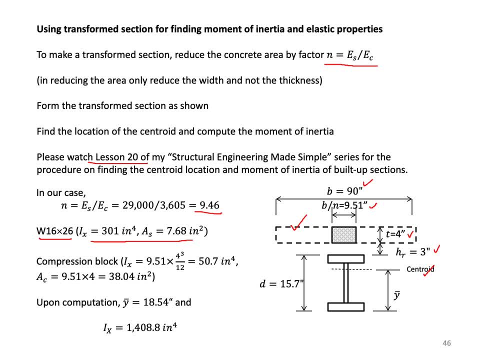 For that compression block. I have its area and the moment of inertia. Using the procedure in lesson 20, I come up with a location of the centroid from the bottom at 18.54, and I get the moment of inertia as this much.